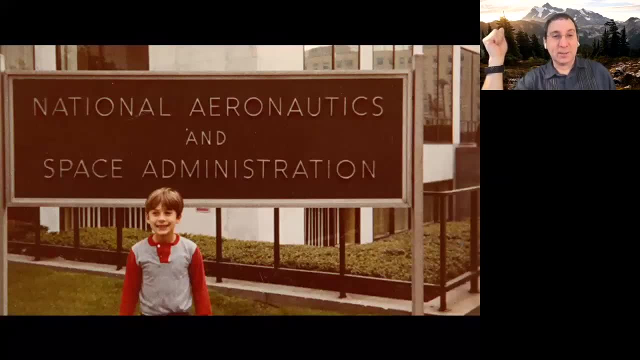 I went to DC, even though I lived in California. And some kids want to go to the Air and Space Museum. I just wanted to stand in front of NASA headquarters. No, I don't know. This is, I think I'm 9 or 10 years old. I had an aunt and uncle that live in Reston, Virginia. They still do. So I got to visit DC a few times. Here's little nerd Shane standing in 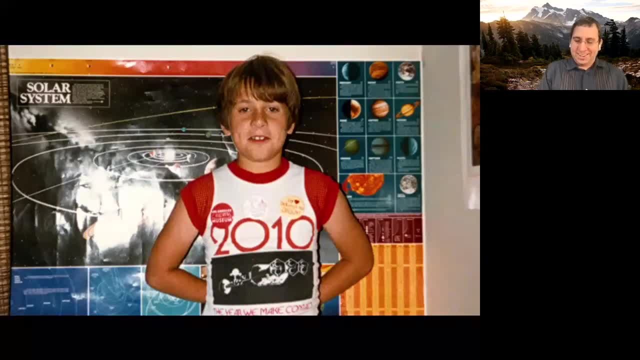 front of his solar system poster. And this is, I'm wearing this shirt. That's when 2010 was like way in the future. Like, whoa, we're going to have spaceships and humans going to Jupiter on a regular basis. That's what I thought. Didn't happen. I also didn't anticipate the internet. 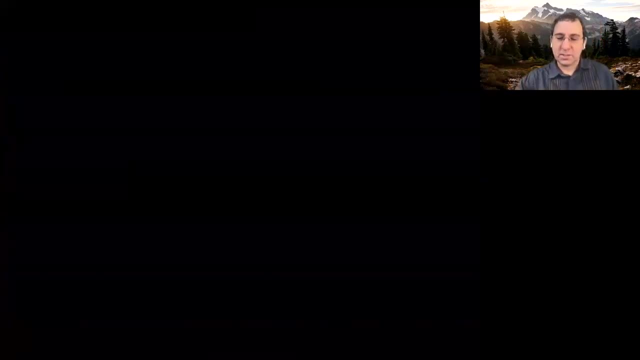 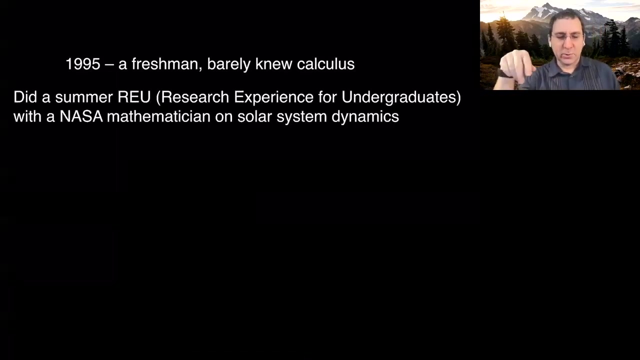 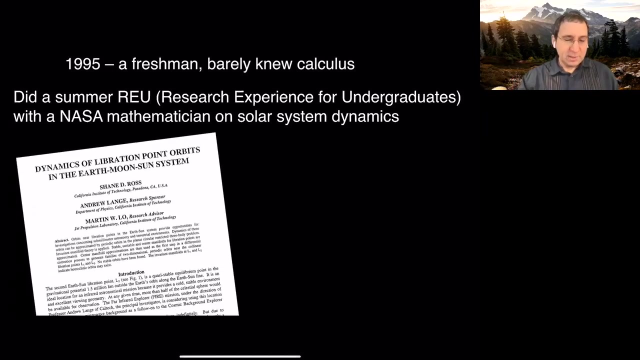 So I got interested in physics. I went to college, took physics. I was a physics bachelor student. I almost failed my first physics class, by the way. Like, almost failed. And when I barely knew calculus, I applied for a degree in physics. And I was like, oh, I'm going to go to DC. I'm going to graduate with a NASA mathematician working on solar system dynamics. I was really interested in like, oh, how do they design trajectories for NASA? You know, they must use relativity or something. And no, they don't. It's just Newton's laws. But I worked with a NASA guy at the Jet Propulsion Lab, JPL. And apparently, I like standing in front of posters. So here's me presenting the work. To a couple of cool dudes. 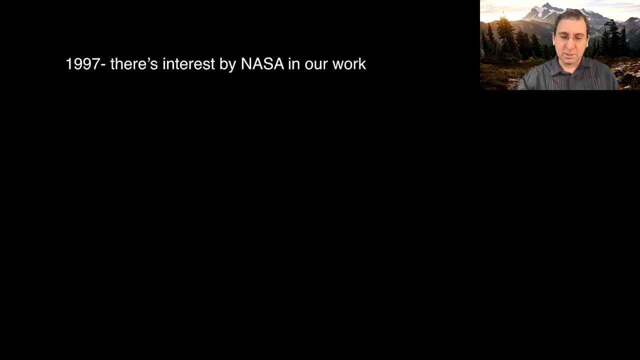 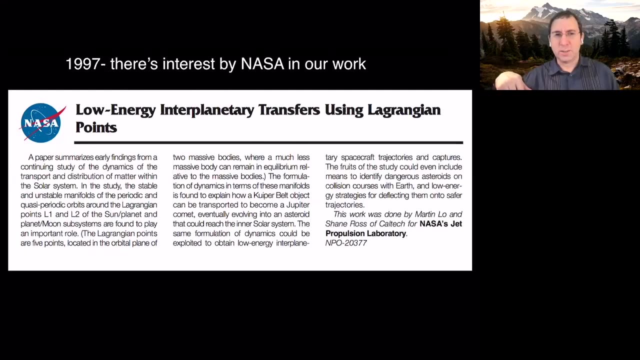 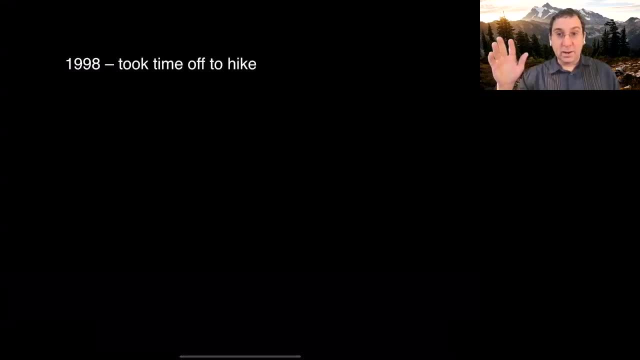 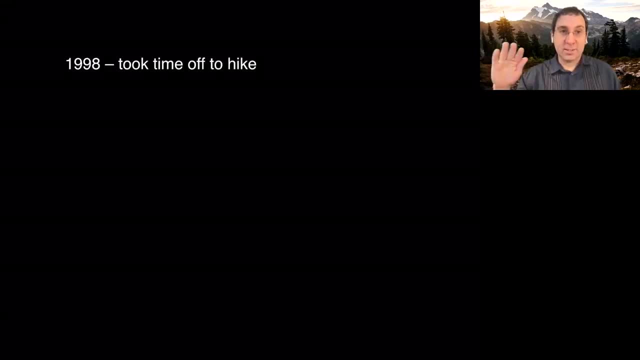 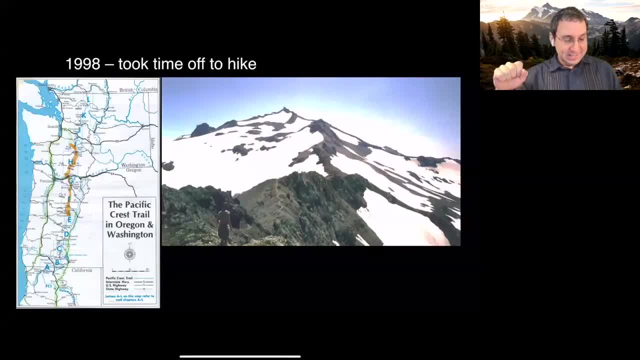 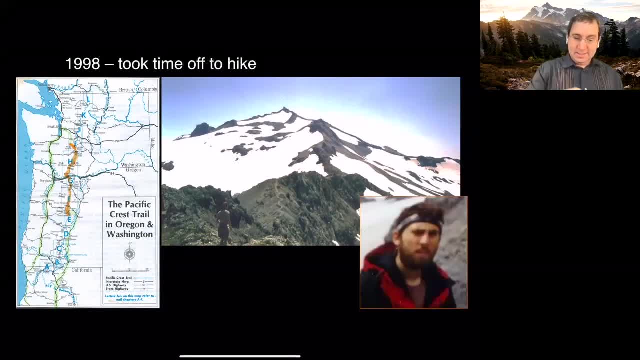 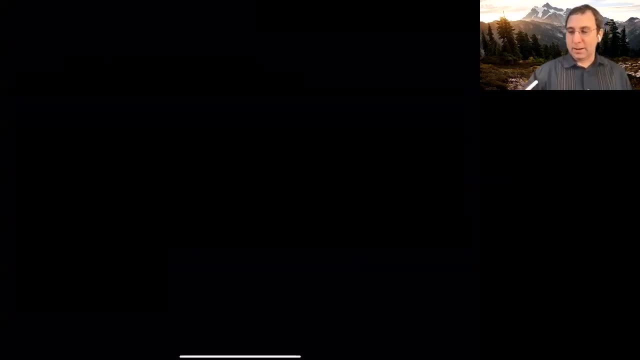 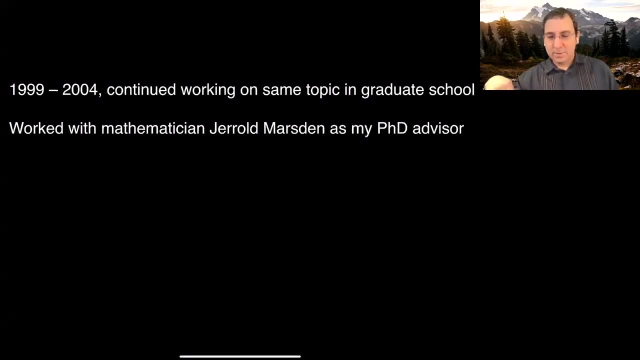 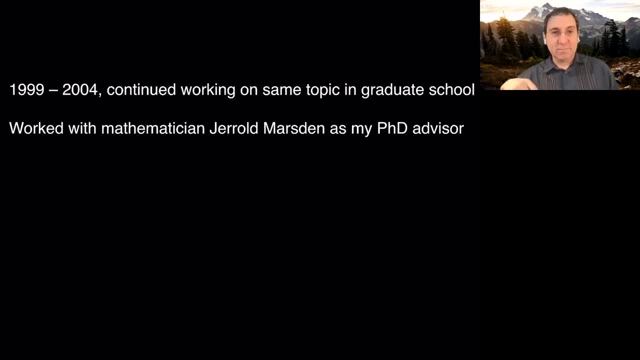 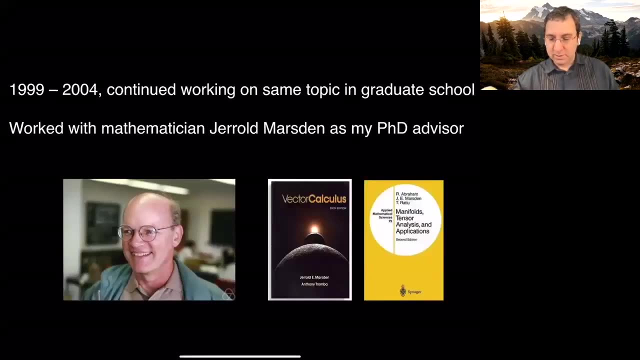 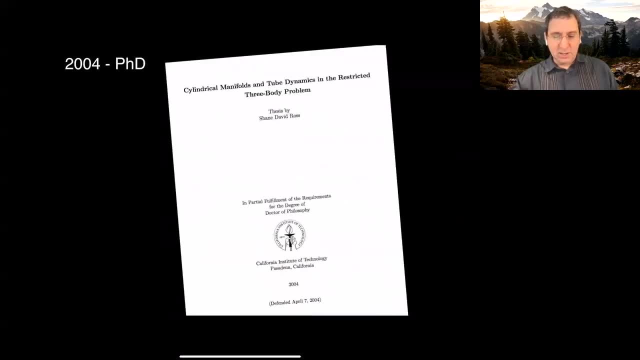 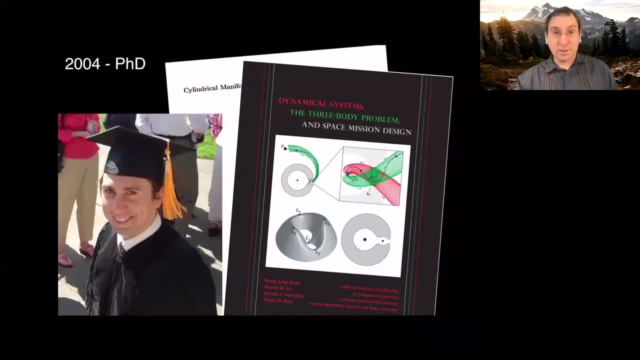 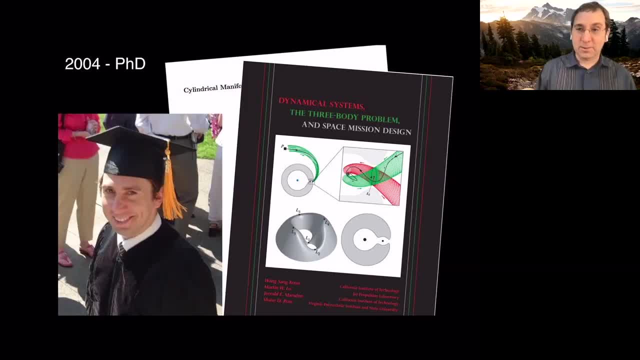 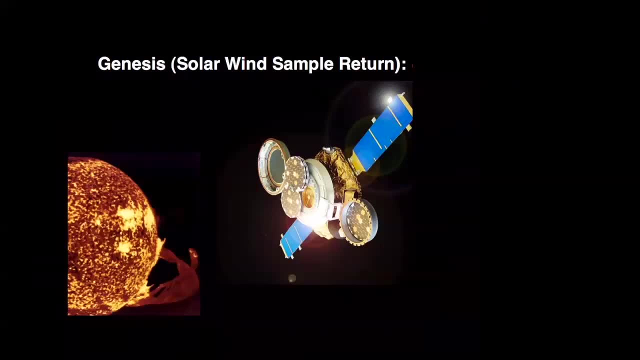 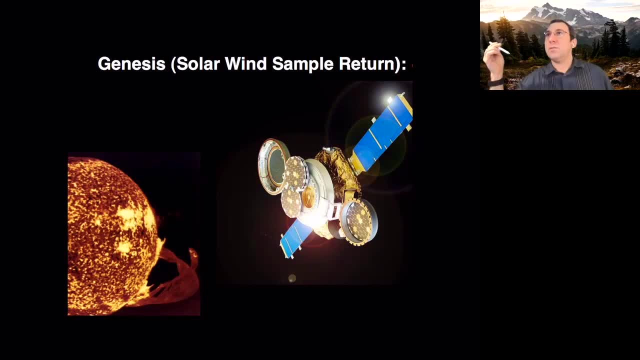 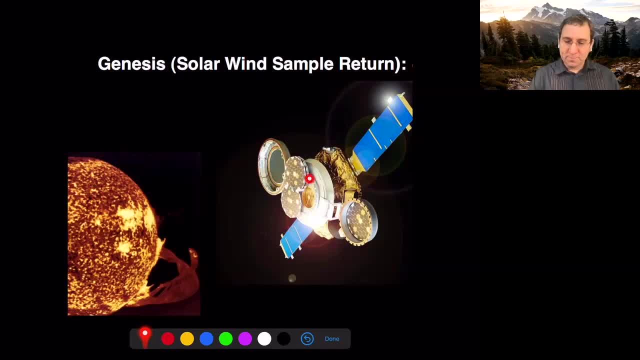 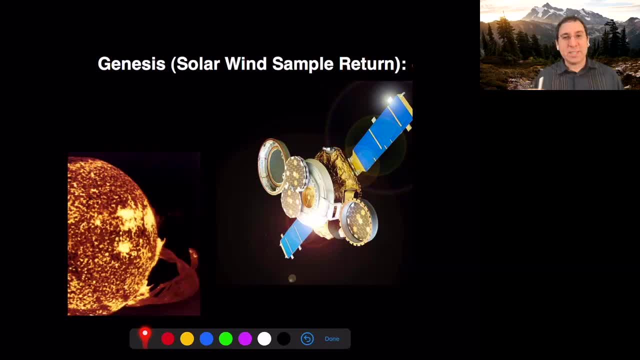 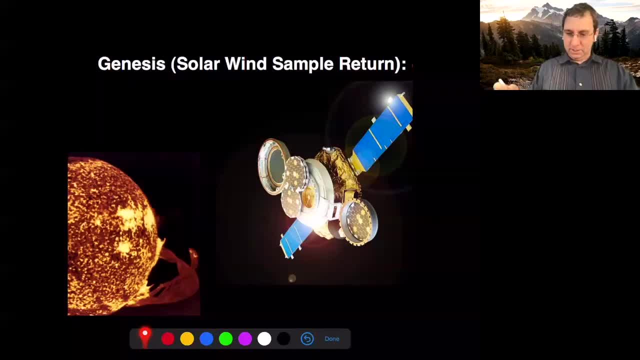 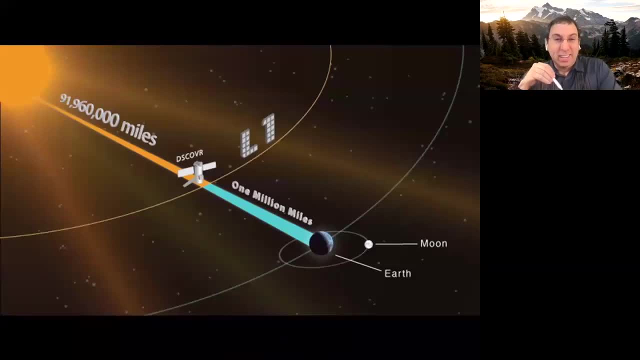 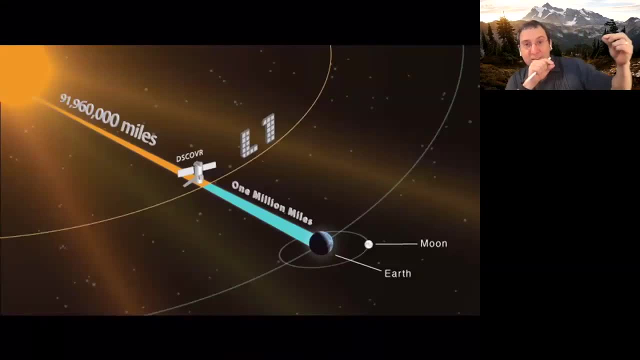 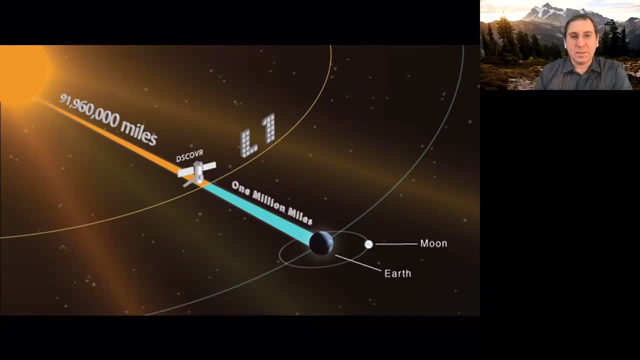 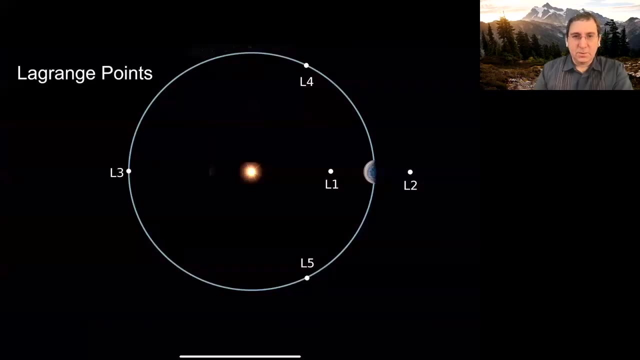 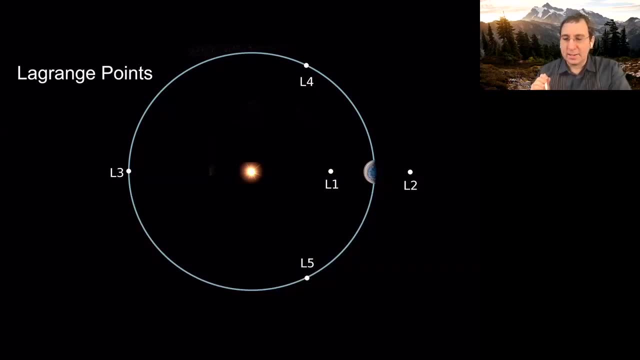 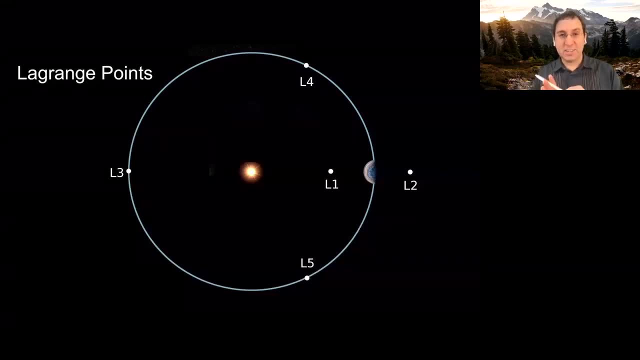 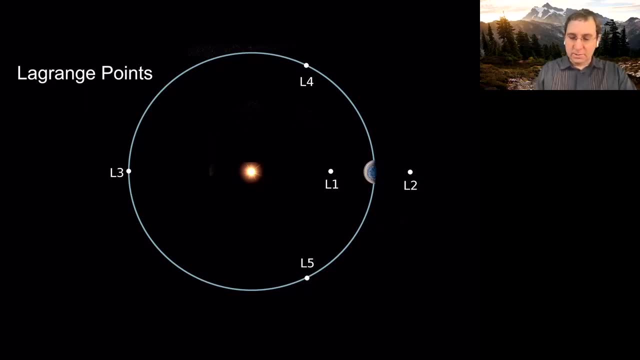 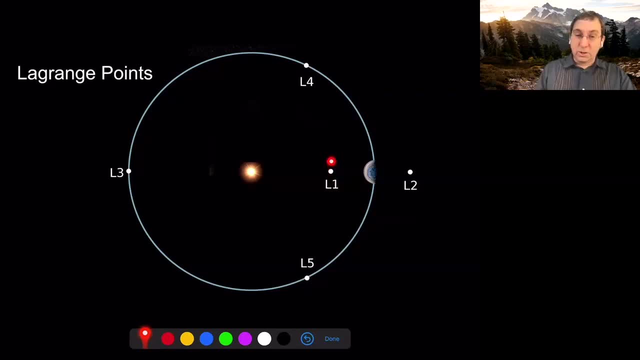 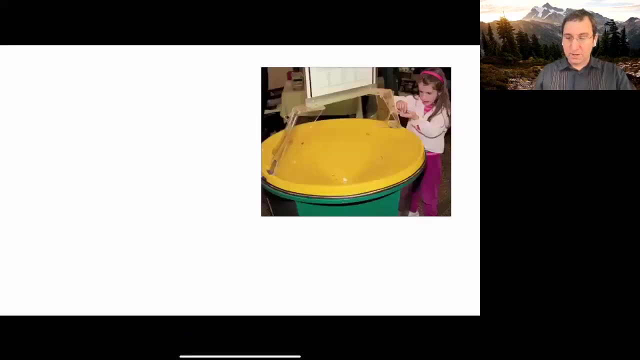 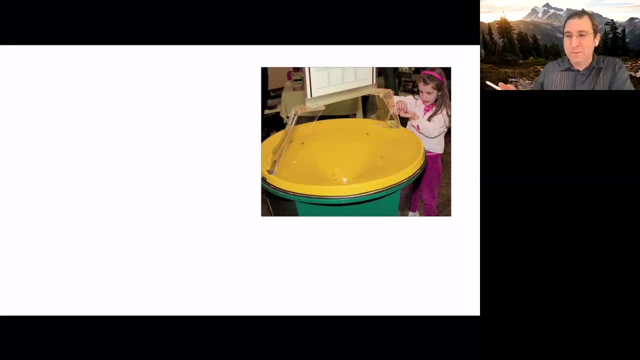 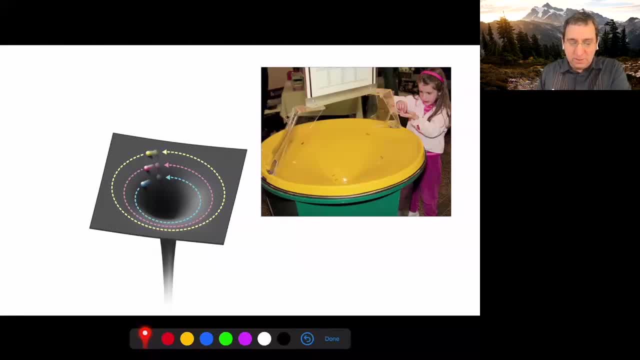 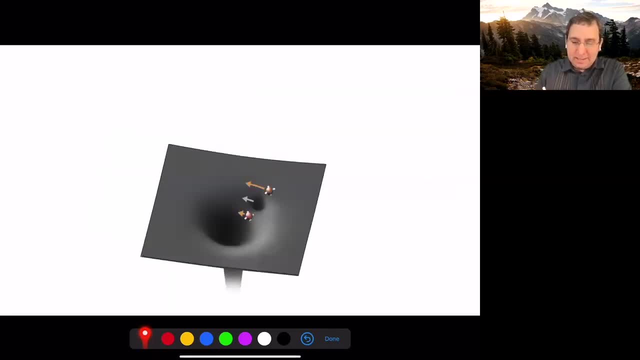 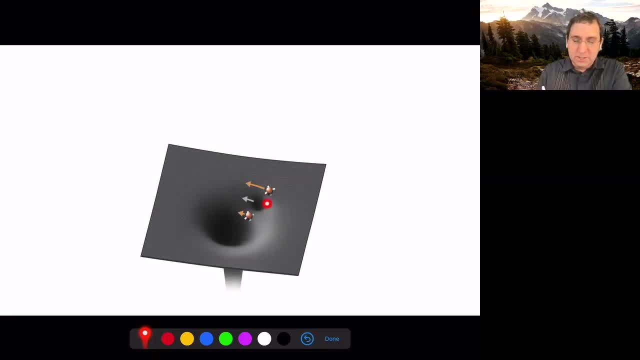 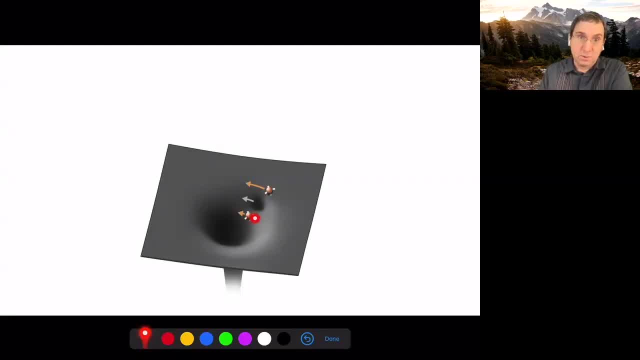 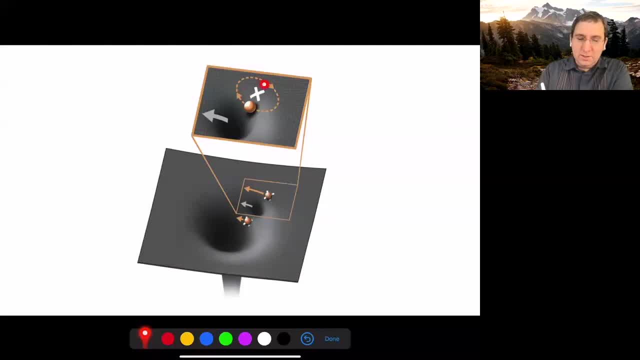 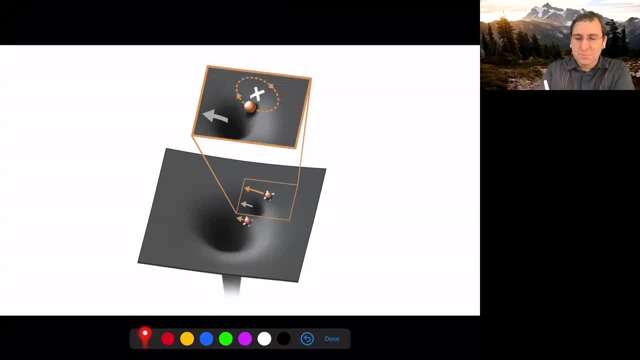 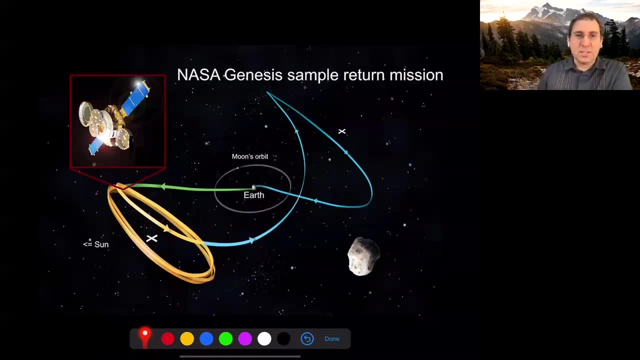 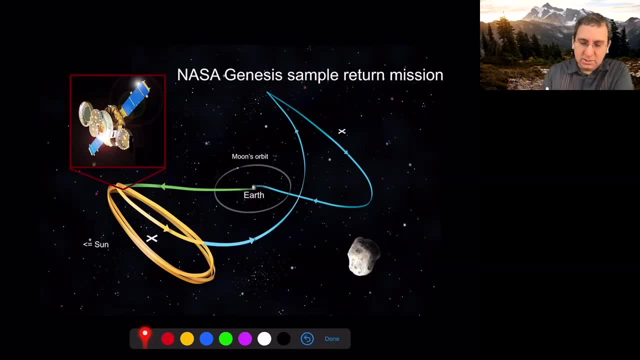 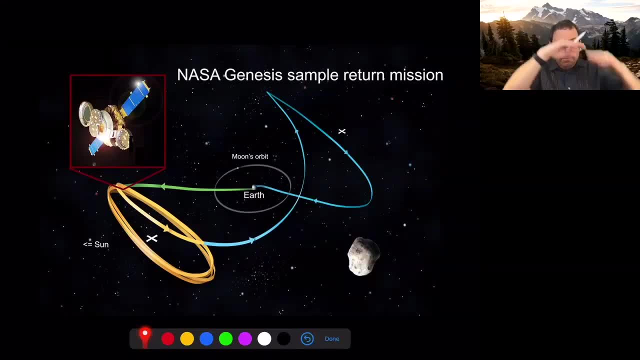 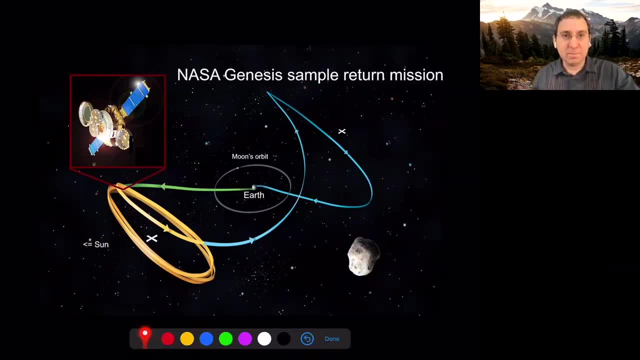 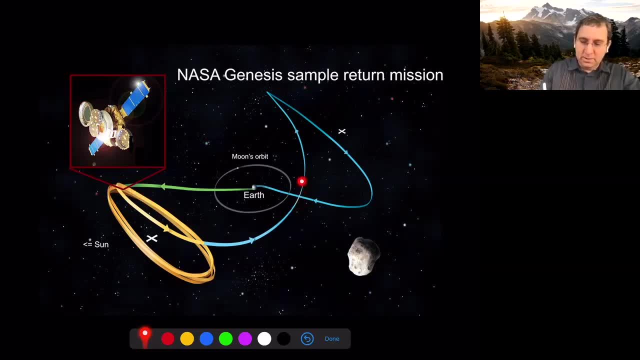 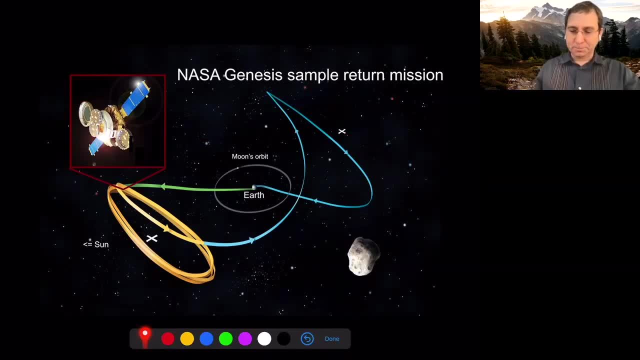 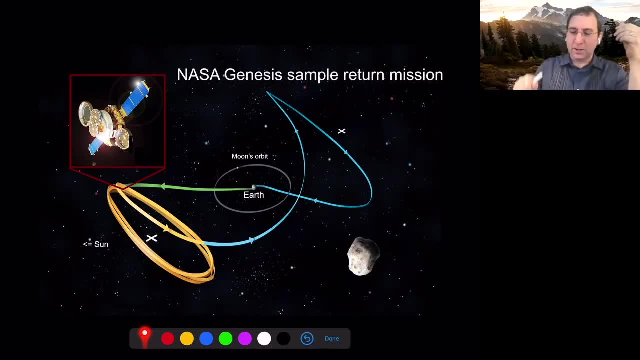 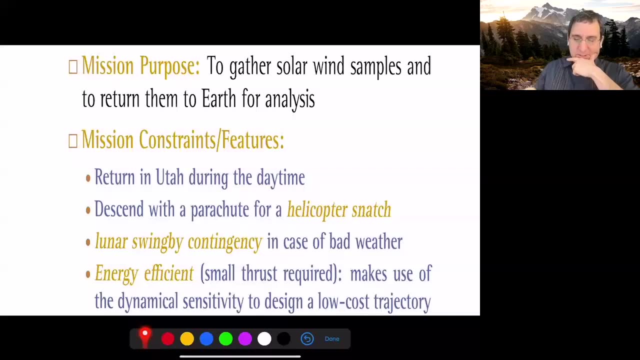 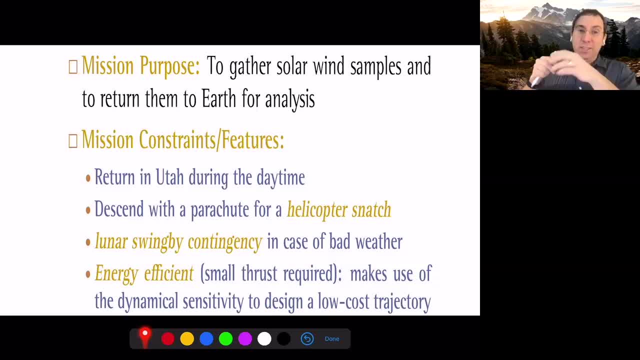 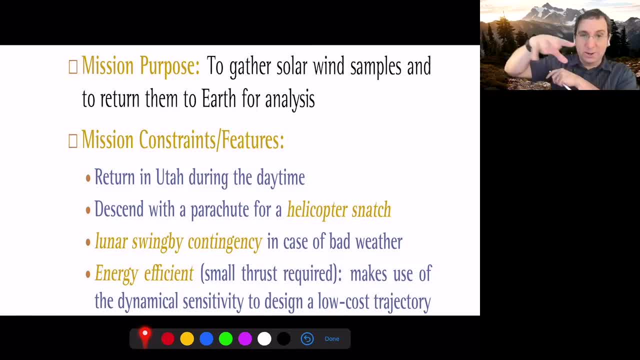 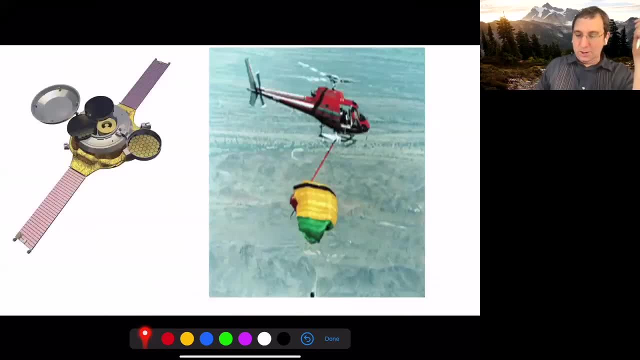 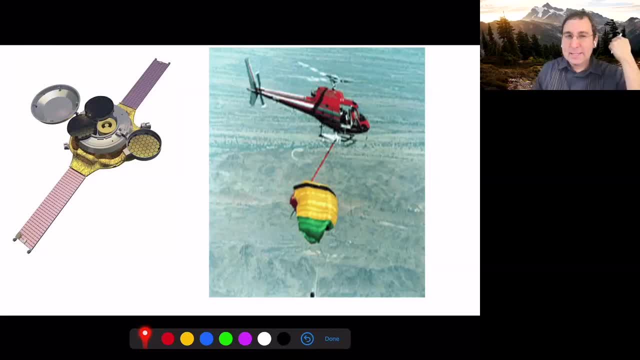 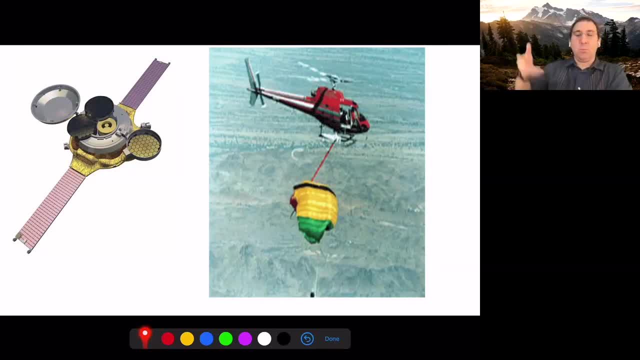 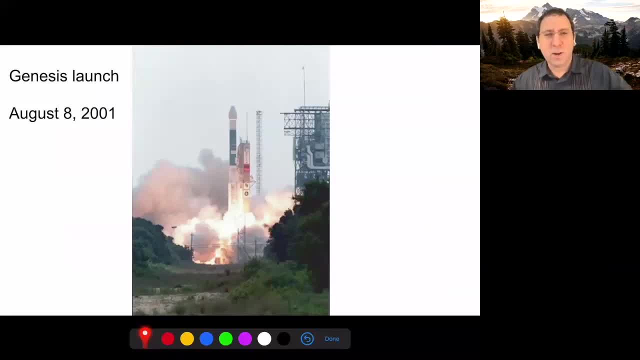 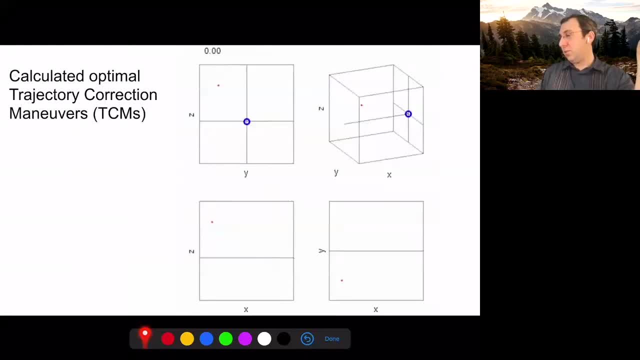 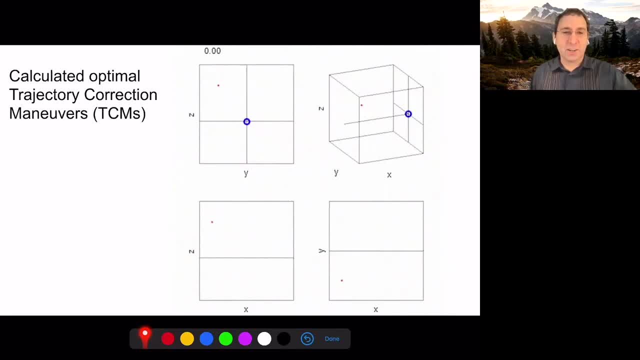 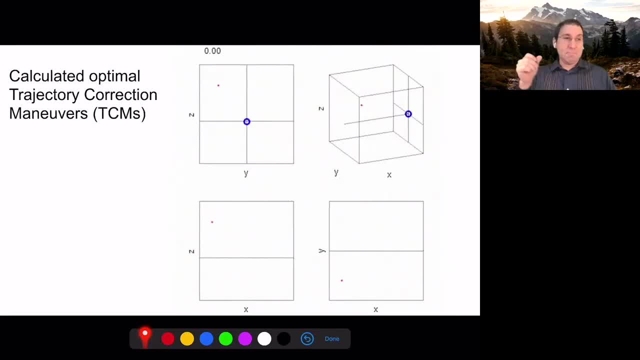 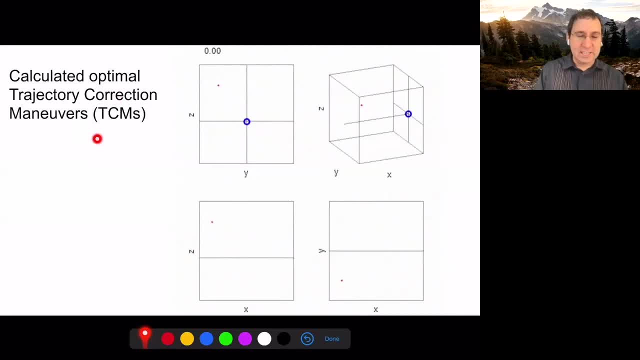 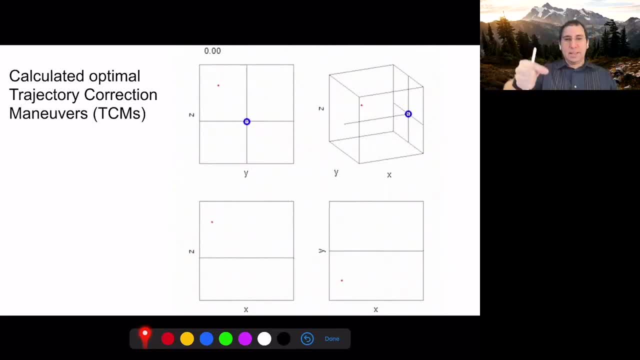 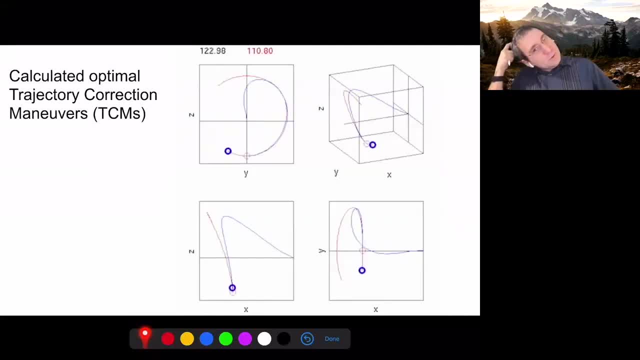 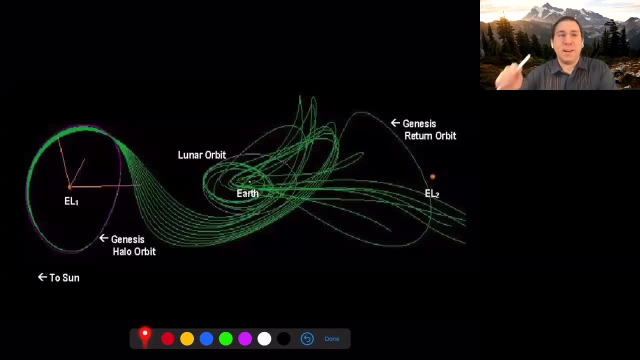 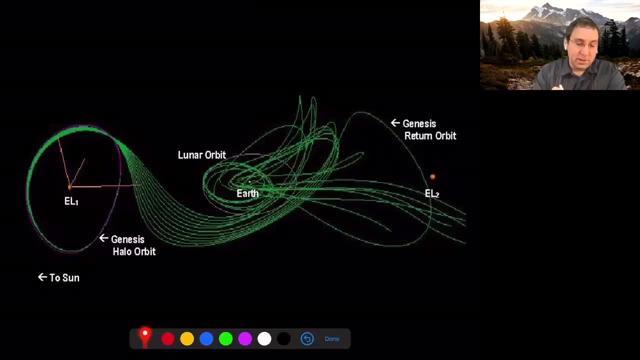 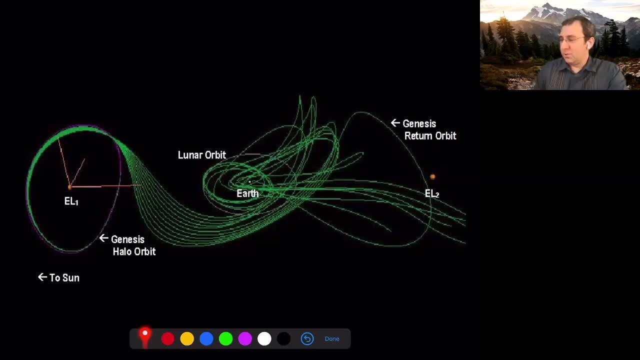 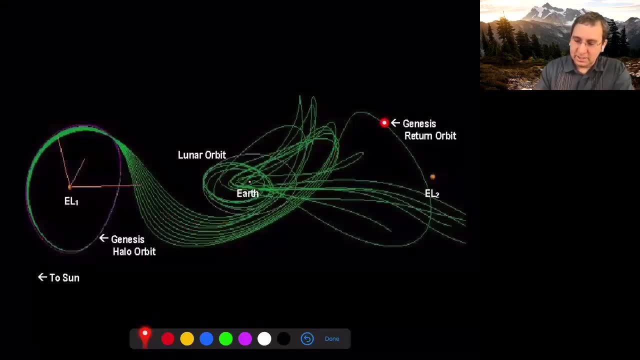 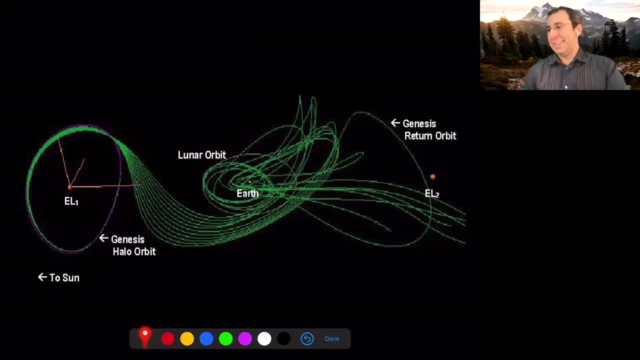 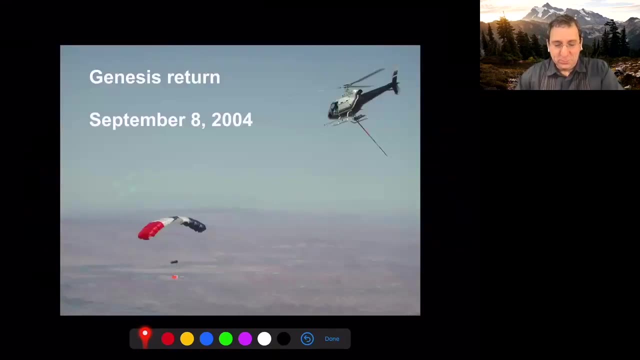 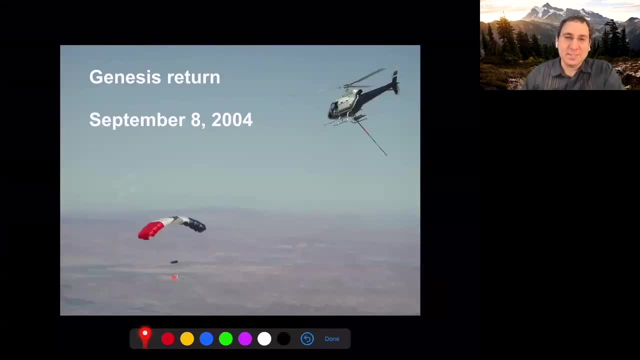 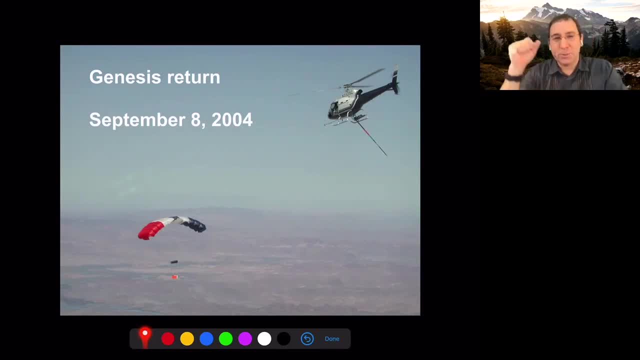 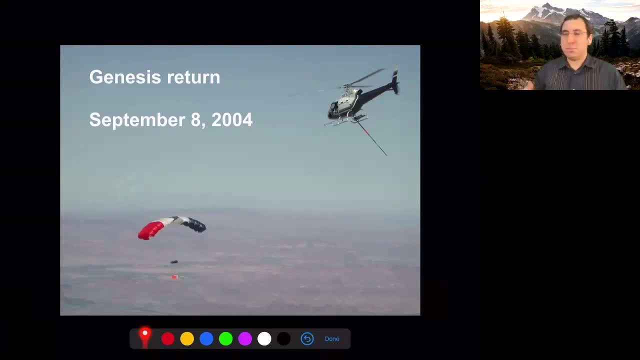 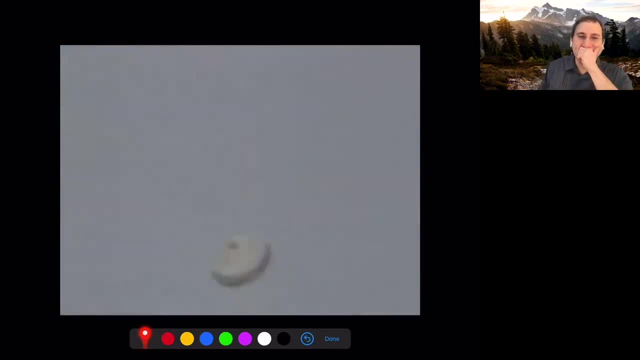 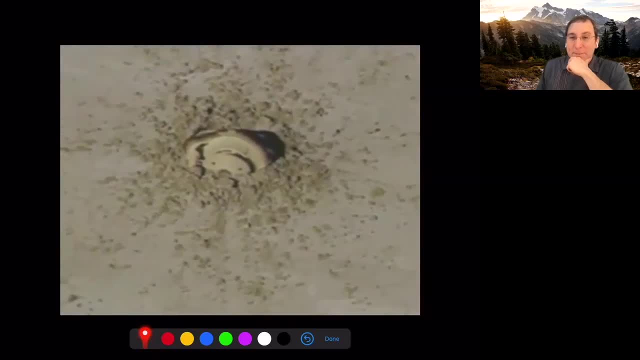 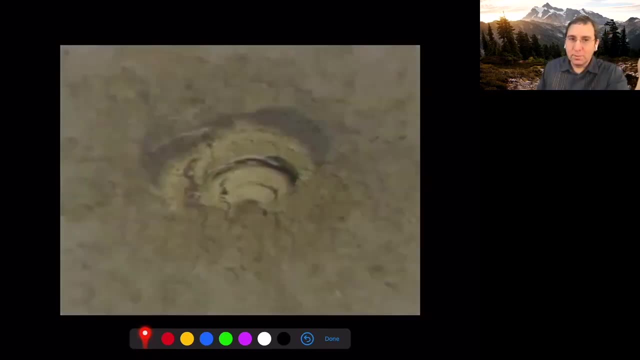 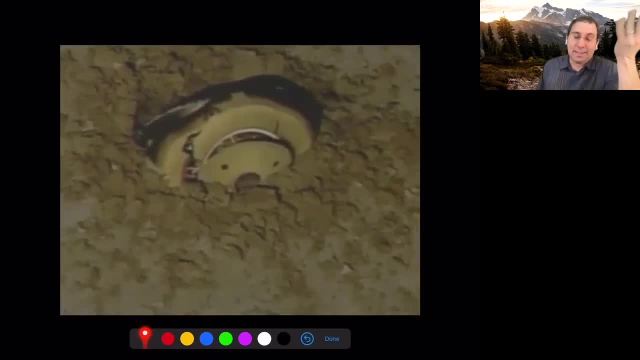 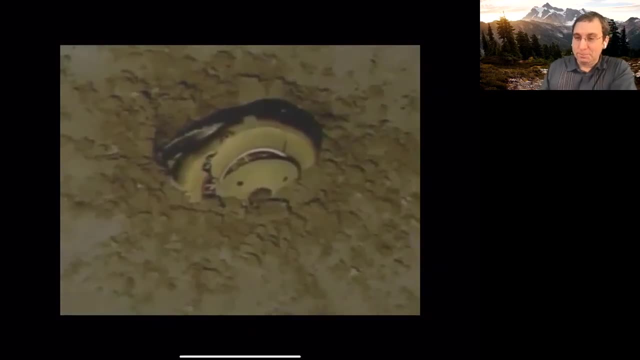 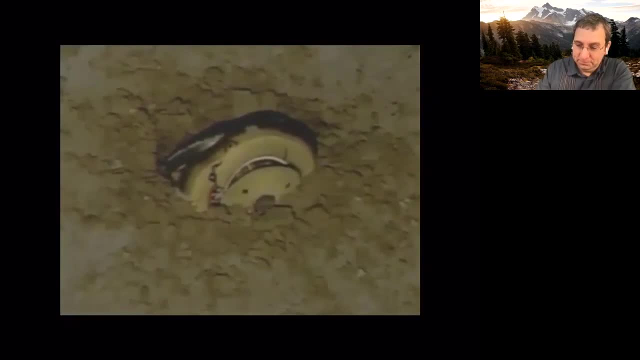 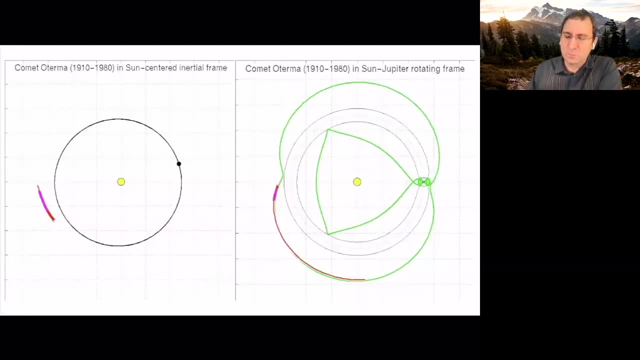 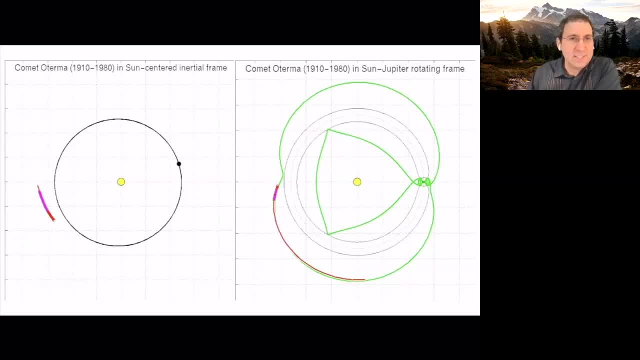 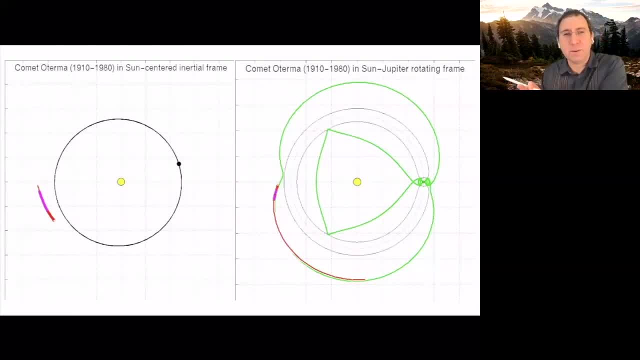 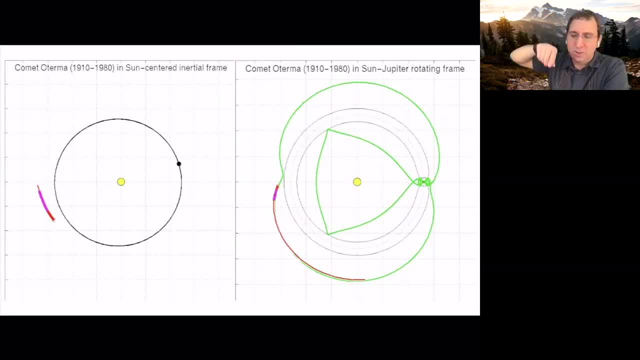 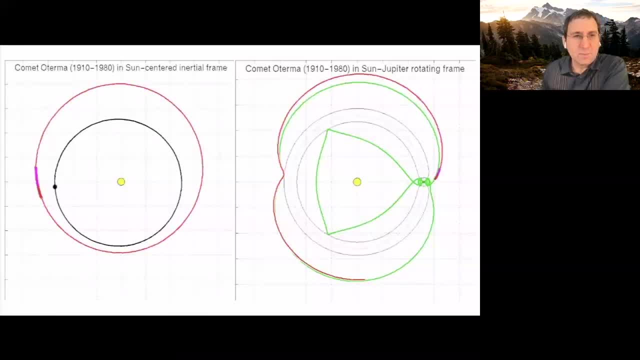 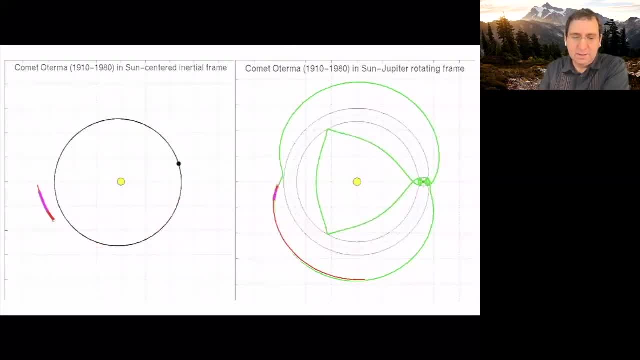 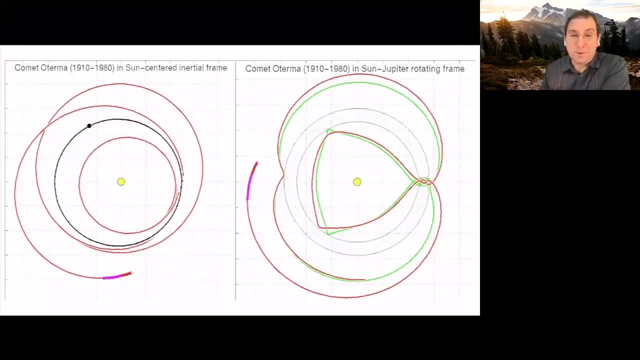 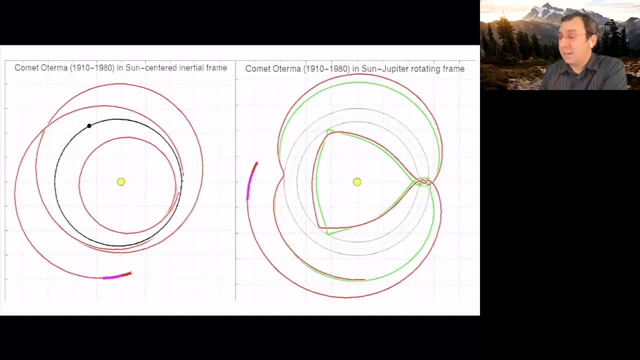 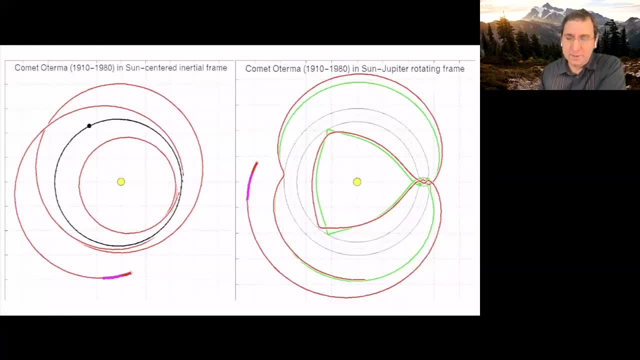 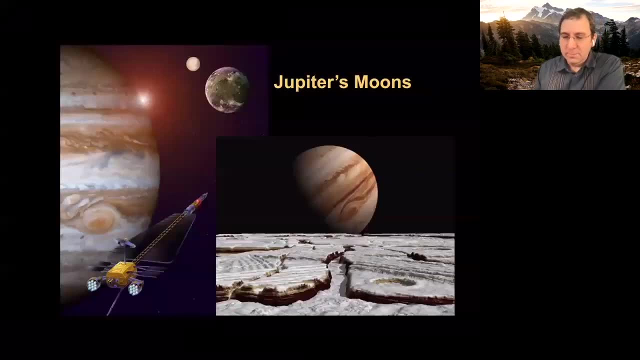 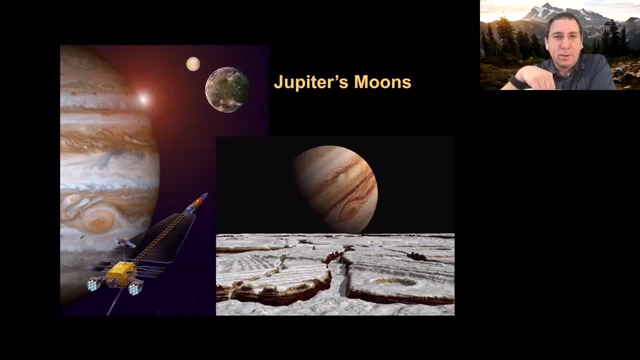 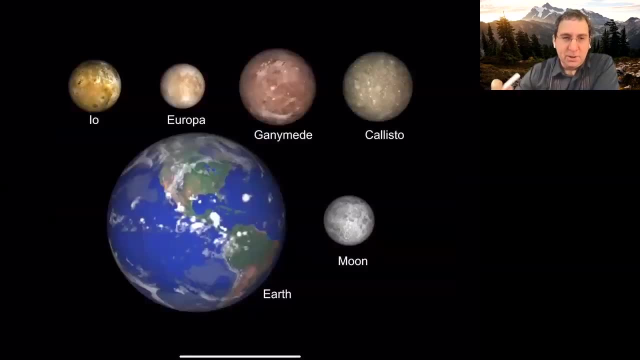 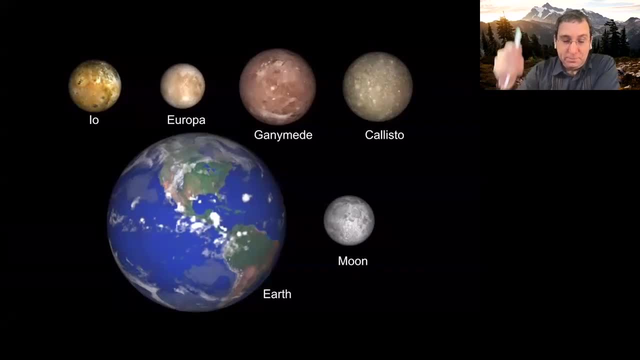 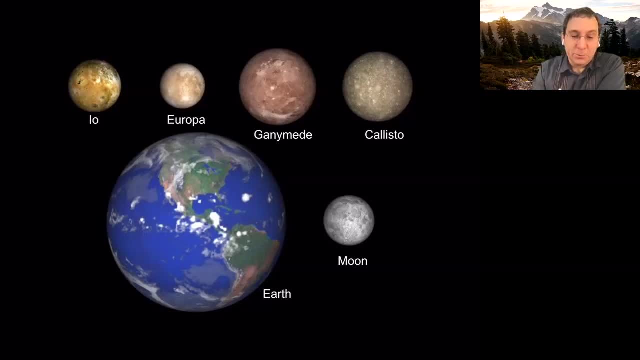 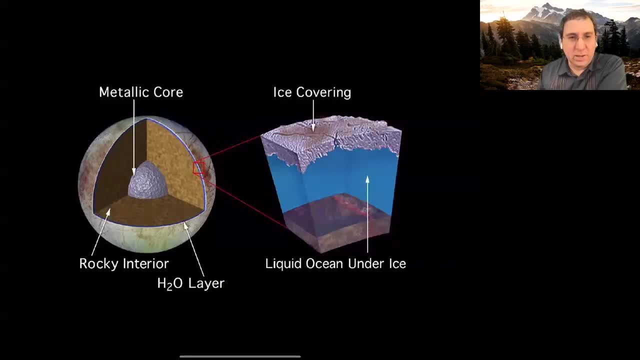 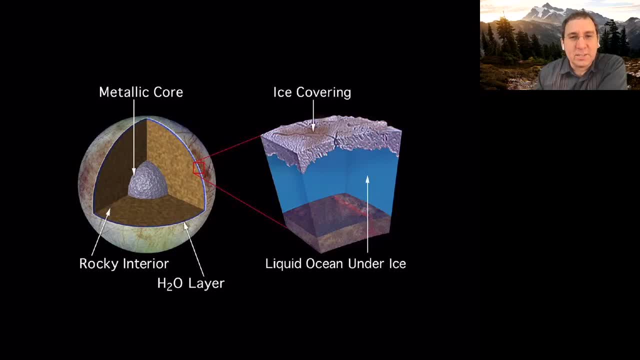 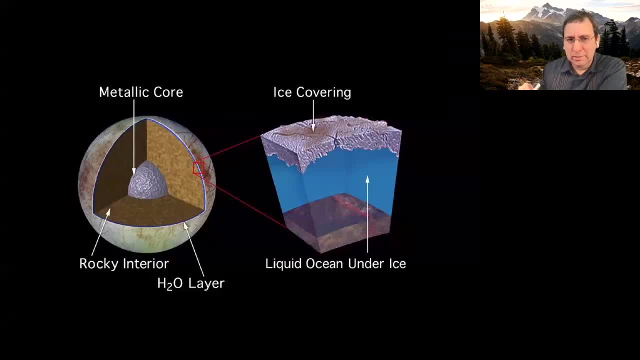 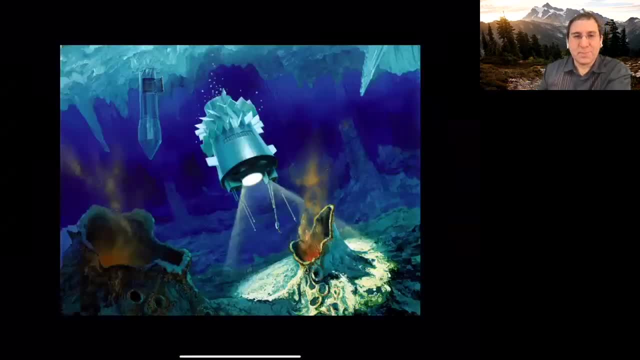 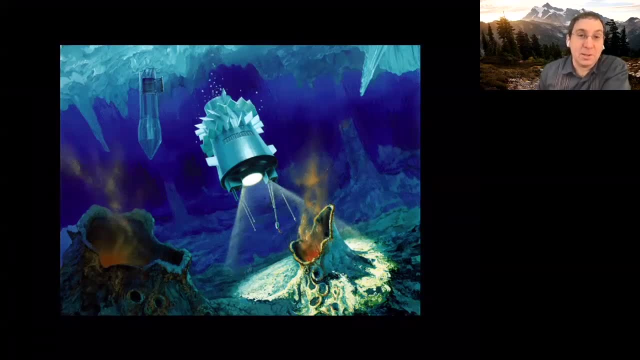 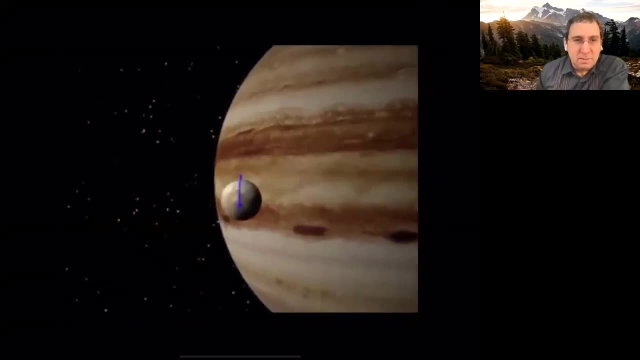 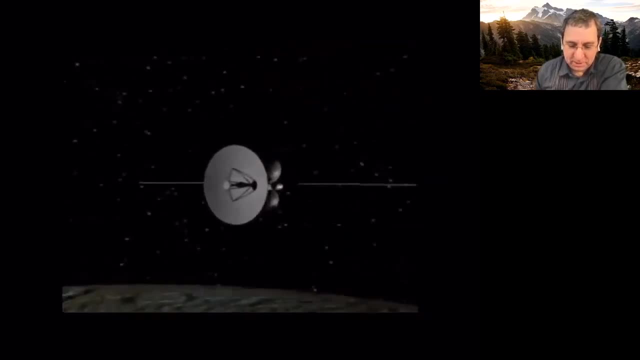 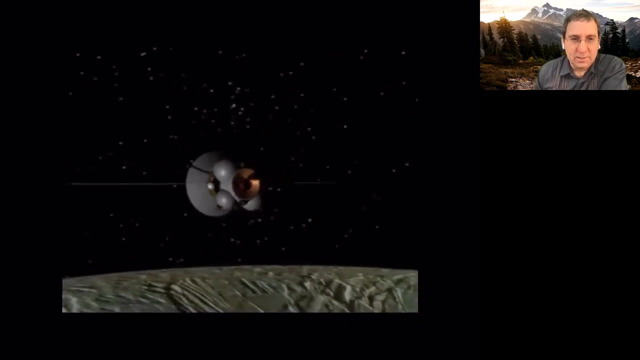 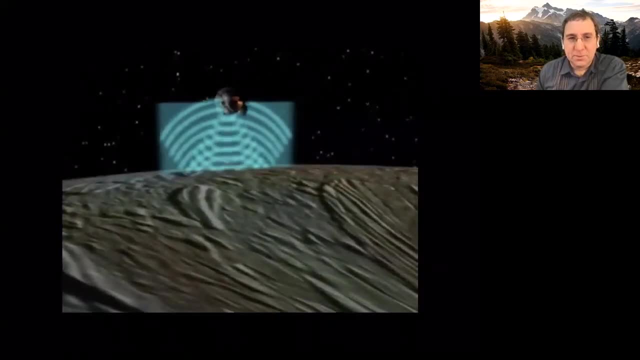 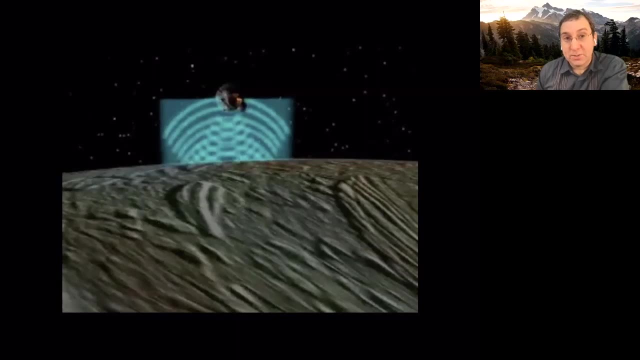 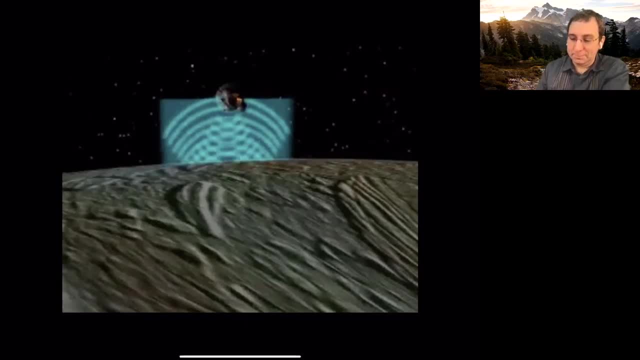 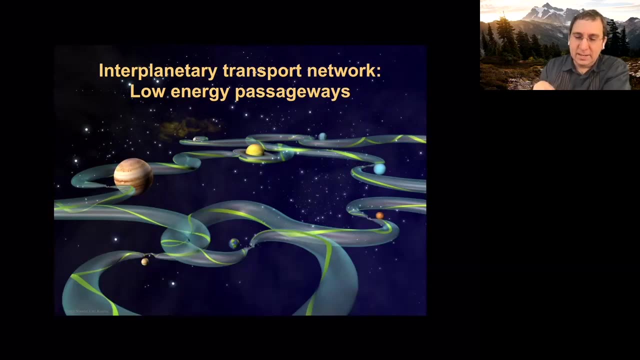 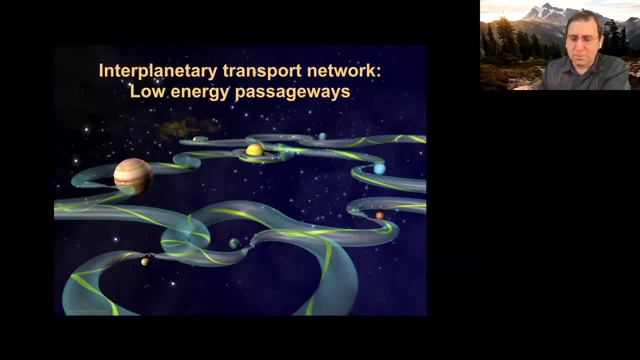 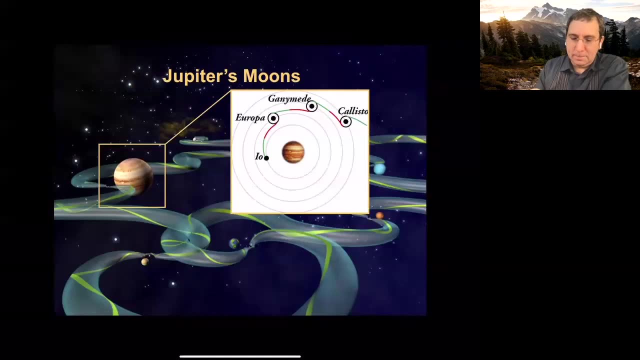 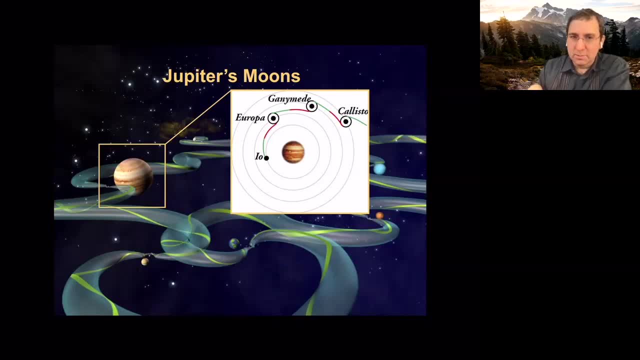 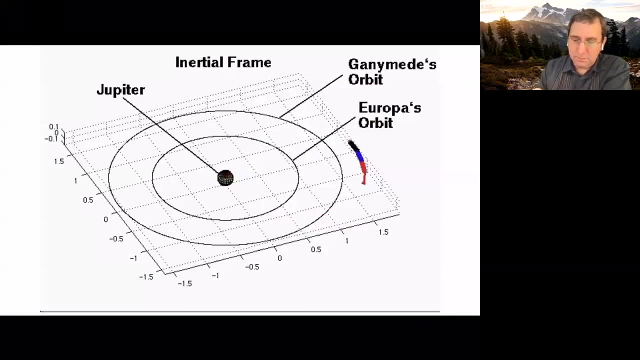 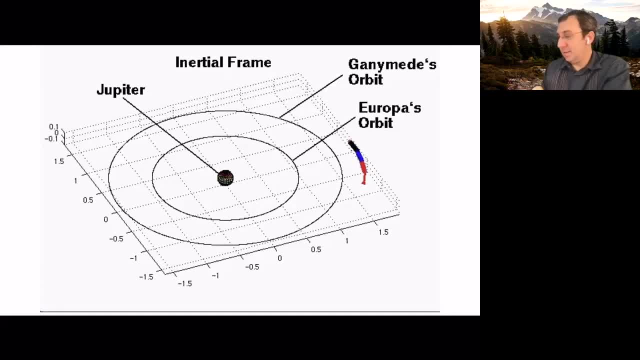 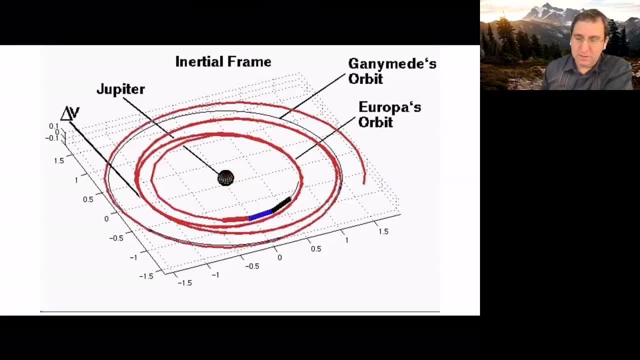 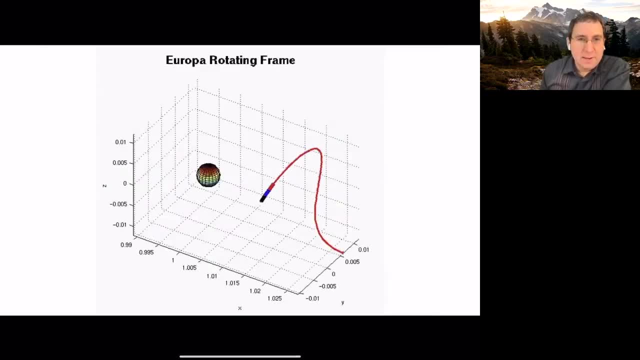 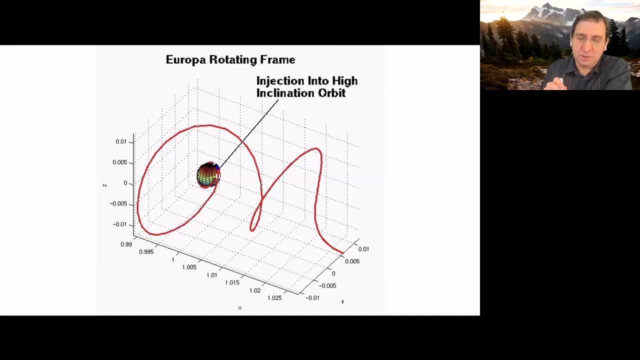 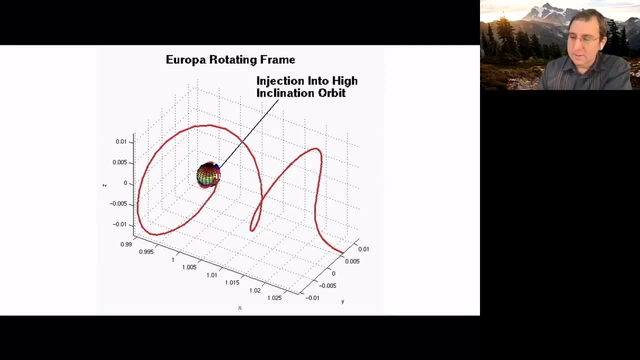 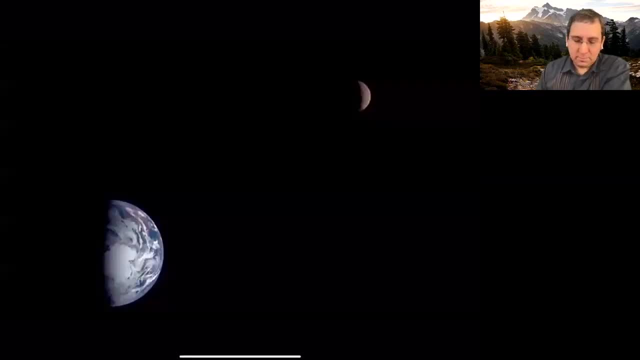 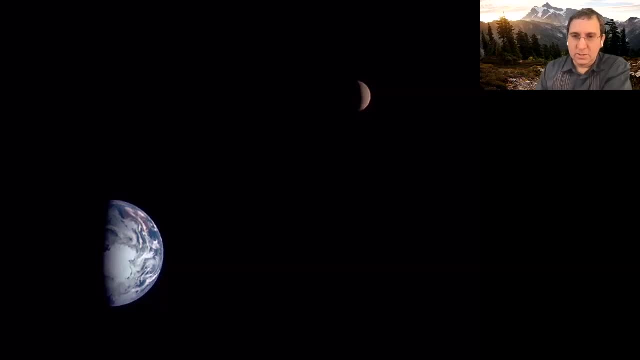 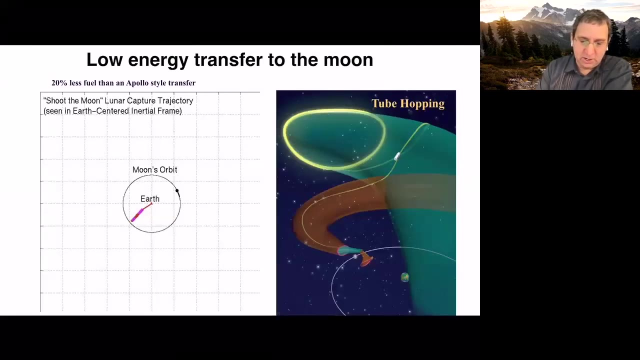 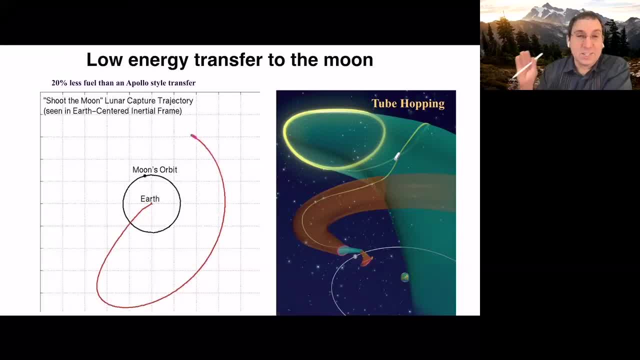 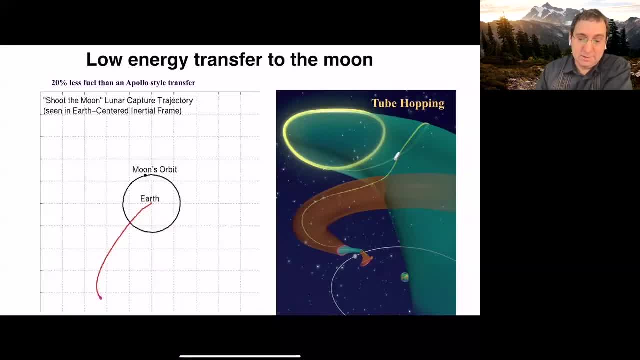 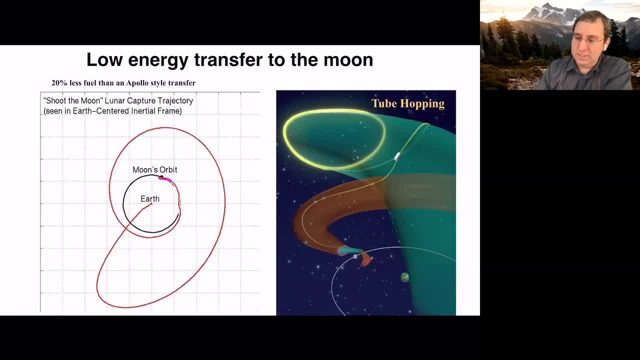 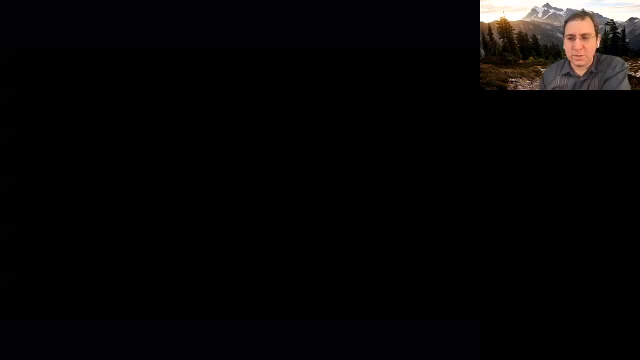 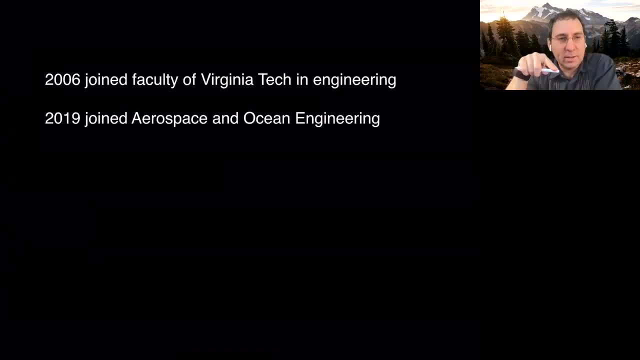 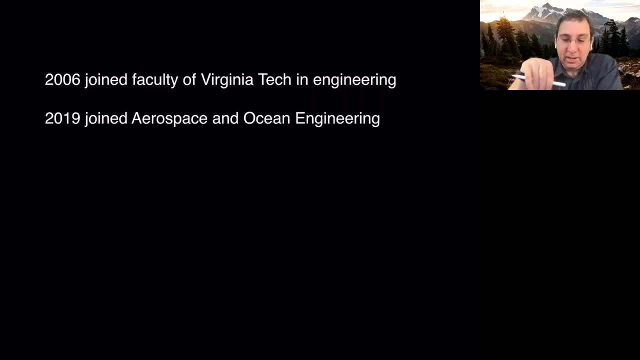 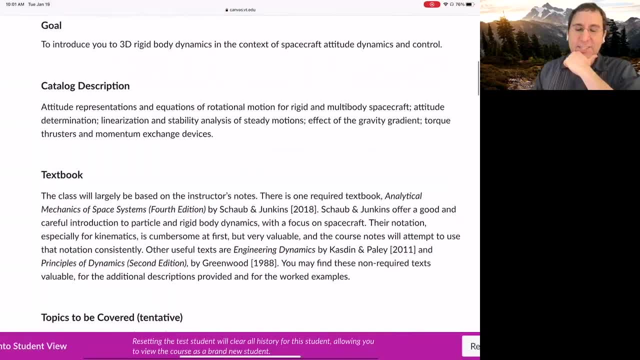 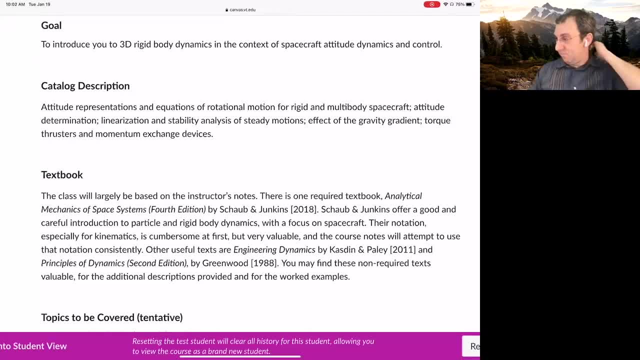 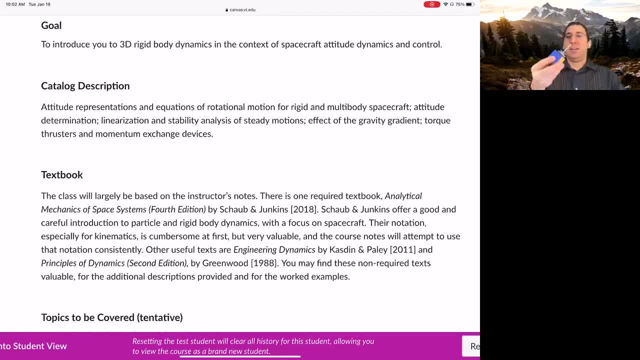 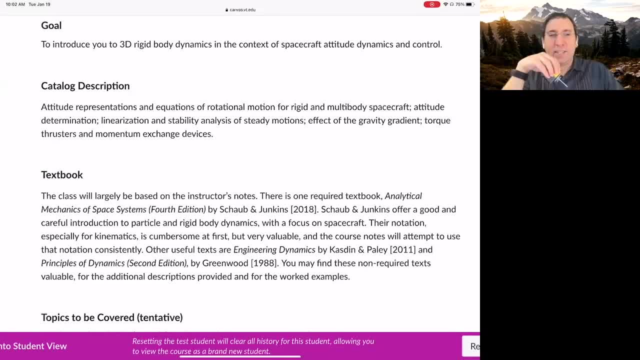 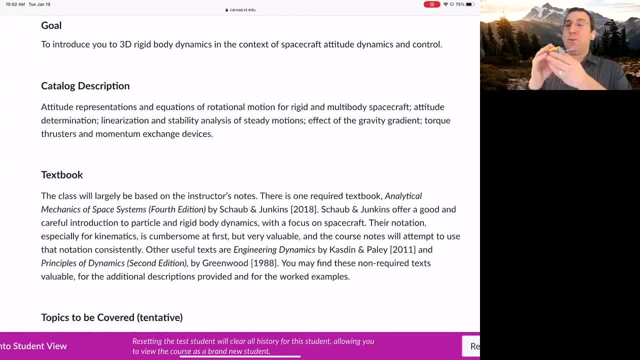 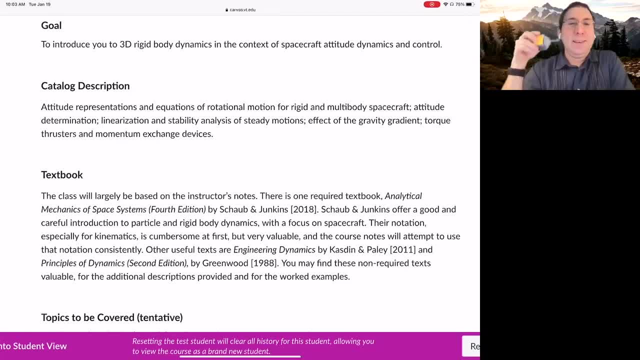 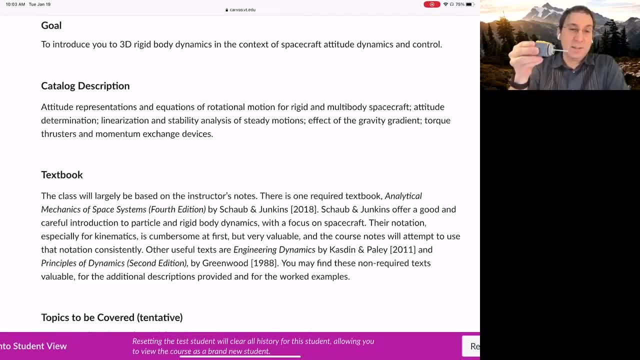 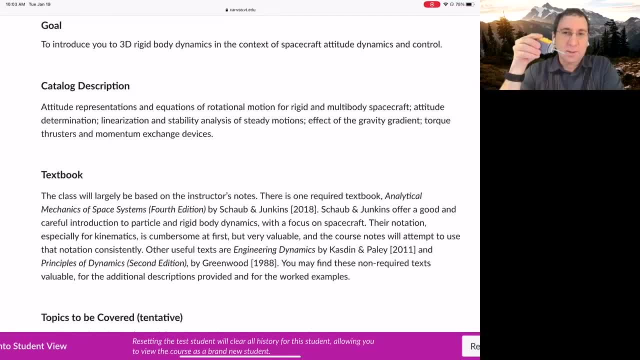 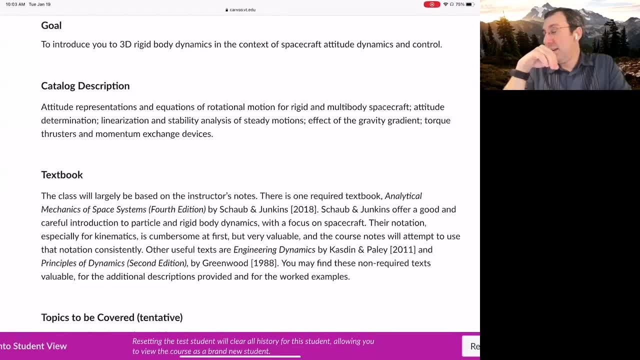 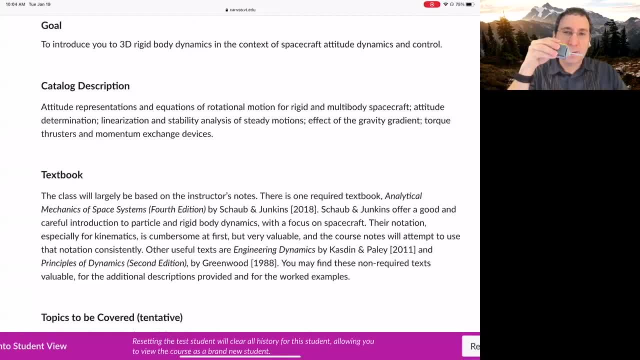 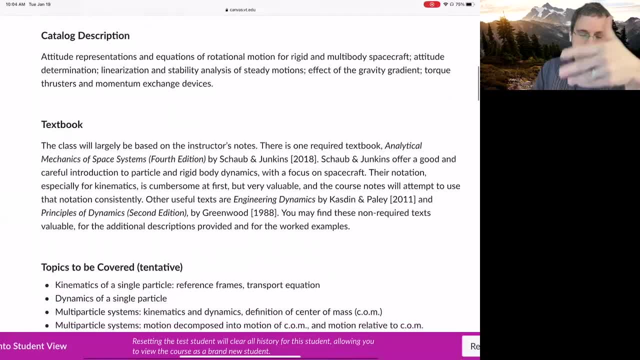 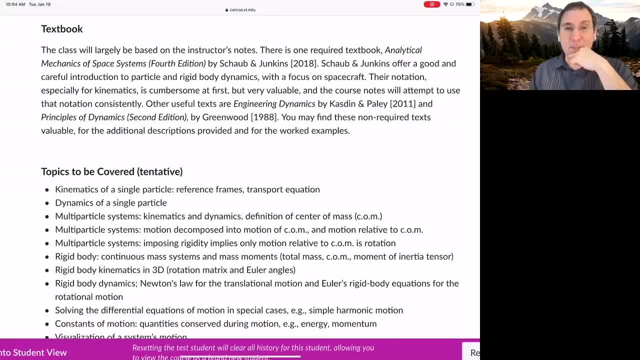 textbook. So this is largely going to be based on my notes, but there's also a required book, Analytical Mechanics Space Systems. I've got it here. It's fourth edition in 2018. It's in the bookstore. It's written by Hans-Peter Schaaf and John Junkins. I know these two. John Junkins is at Texas A&M, and he's a nice guy. And one of his PhD students was Hans-Peter Schaaf, who was actually at Virginia Tech until about 2007, and then went to University of Colorado. 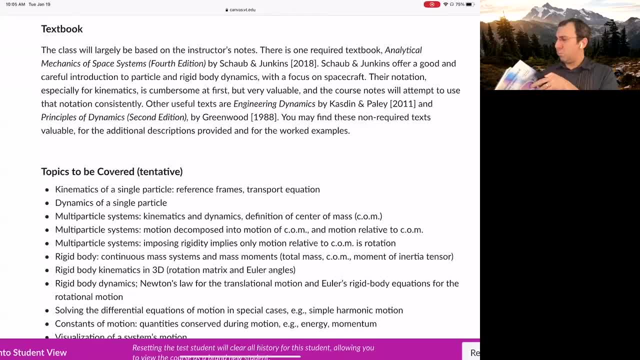 So they wrote this book, and I think we're mostly just going to be looking at the first four chapters. There's other books that take, which is like half the book. There's a lot of books that take half the book. There's a lot of books that take half the book. There's a lot of books that take half the book. 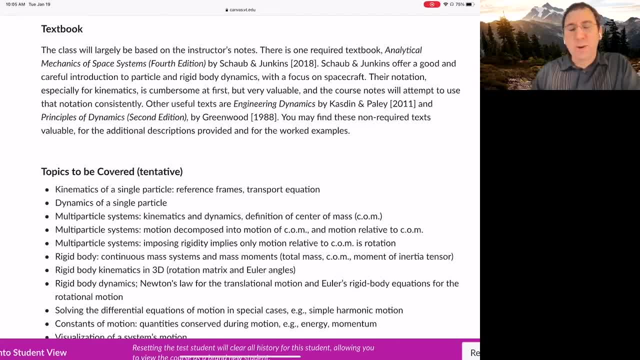 There's other books that take too long. I would rather stick with the keep it simple 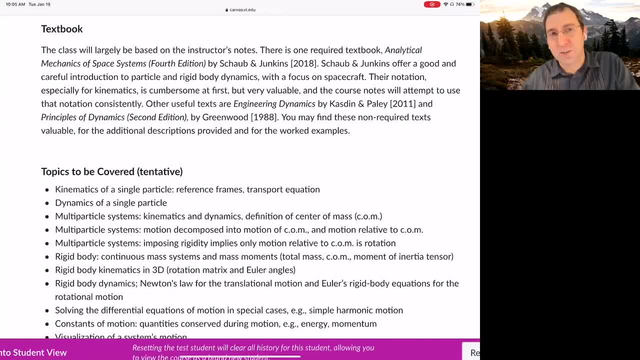 principle. So I'm going to try to keep it simple and give you intuition as much as we can. There's other textbooks that are not required, but might be useful. So this one is listed right there, 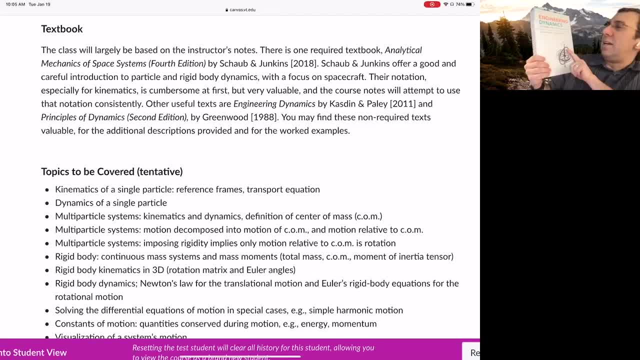 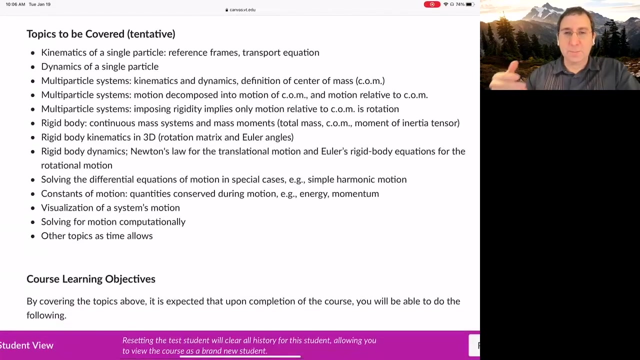 Engineering Dynamics by Kasdan and Paley. They're also from aerospace and mechanical engineering departments. And they use some very similar notation, but I will be sticking with the notation of this book. They're very careful about writing the kinematics because that is foundational. And then there's this other book, Principles of Dynamics by Greenwood. I don't have a copy of it here. It's probably in my office. And why look at the other books? Because they have lots of worked examples. In this class, I'll be trying to give you theory, and also working through examples, because that's really useful. Here are the topics that we're going to cover. There'll be some, probably next time, be some motivation on 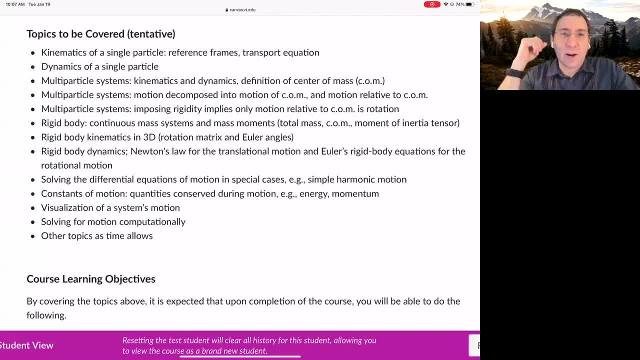 mission analysis and the requirements for pointing, just so that, you know, why are we doing this? But then we'll go into more of the theory about kinematics for a single particle, 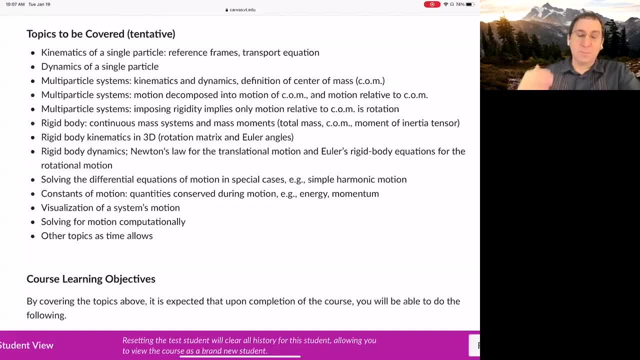 and reference frames. Then dynamics of a single particle, we're going to kind of build up to rigid bodies by talking about multi-particle systems. And then 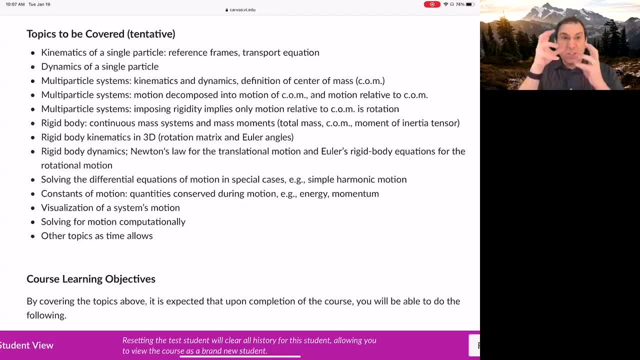 if you have a multi-particle system where all the particles are rigidly attached, that's a rigid body. And then you can think of a continuous mass system. 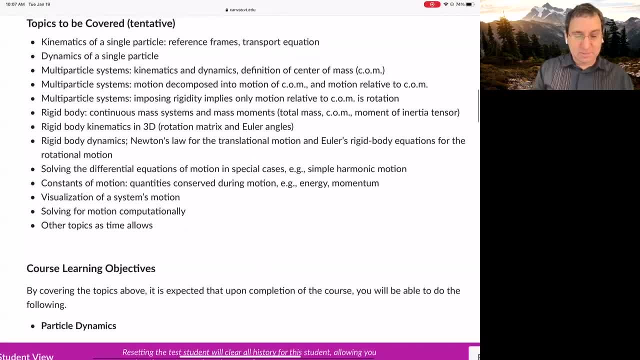 So, we'll talk about rigid body kinematics and then that's just describing the orange. And that's just describing the orientation of a rigid body. Here's a rigid body. 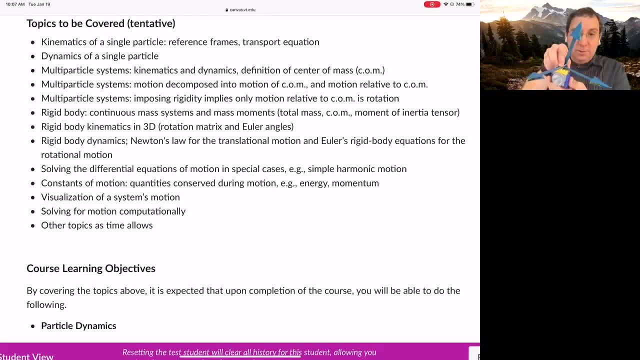 And it basically comes down to attaching a frame. Look at this cool triad of vectors that I made and painted. 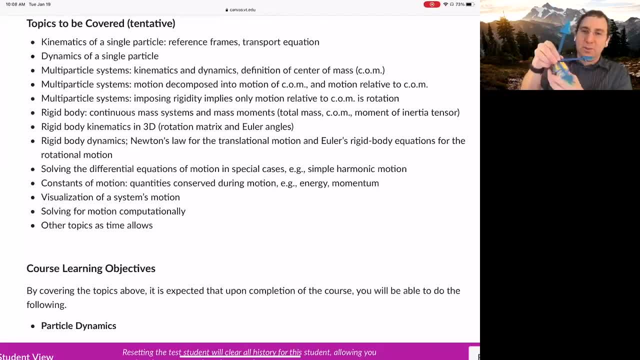 All right, so you're trying to describe how these three vectors that describe a frame attached to your body, how do they change with respect to another frame, an inertial frame? And that will be a big part of what we do. 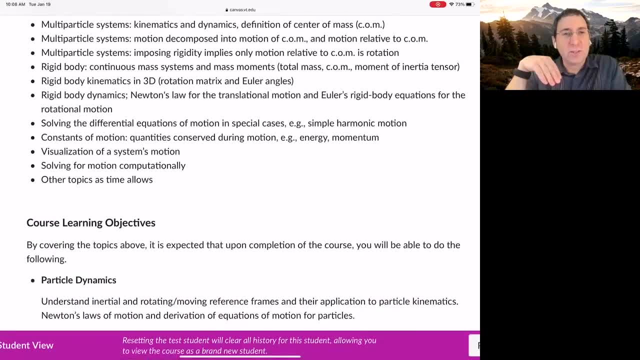 And then eventually, once you have some dynamic equations, you can solve these analytically in simple cases or special cases. 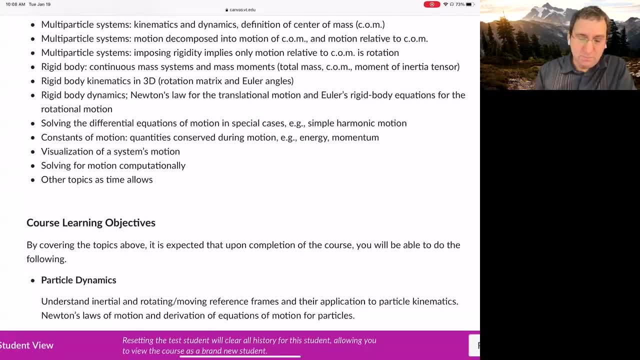 And then there's constants of motion, like energy and momentum, and that's all good. 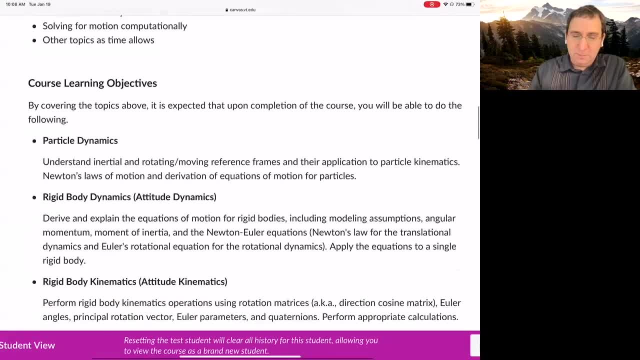 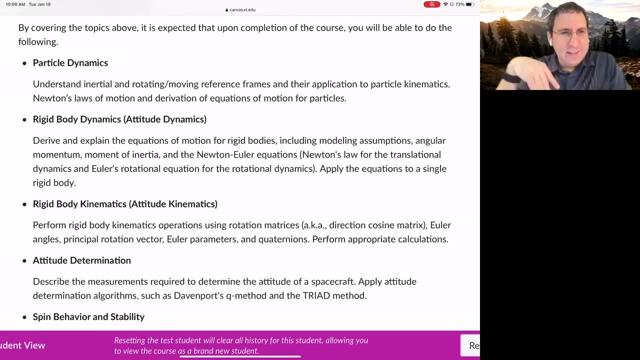 All right, so covering those two topics above, you should be able to do the following. You'll be able to understand inertial and rotating reference frames and how they relate to particle kinematics, and then use Newton's laws to derive equations of motion for particles. 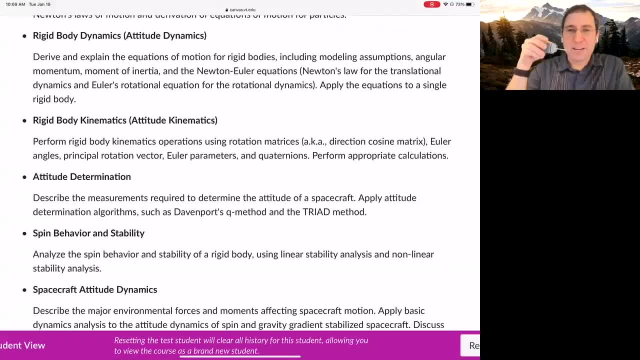 Rigid body dynamics are, for spacecraft, the terminology seems to be attitude dynamics. 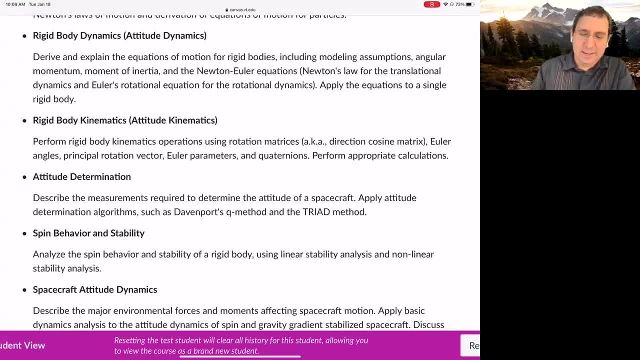 So derive and explain the motions of rigid bodies. So derive and explain the motions of rigid bodies. So derive and explain the motions of rigid bodies. 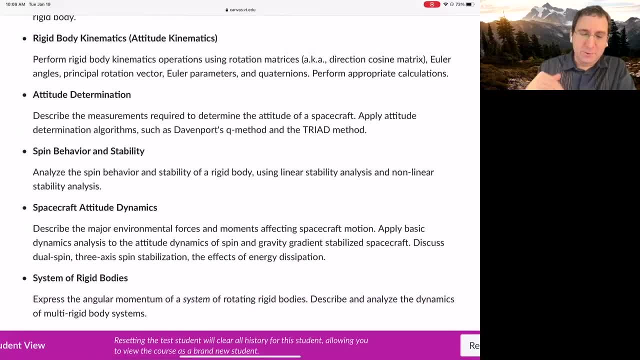 And even before that, there's rigid body kinematics that describes the orientation of the rigid body. And a big part of that will be rotation matrices and other ways of writing a rotation matrix in terms of angles, quaternions. 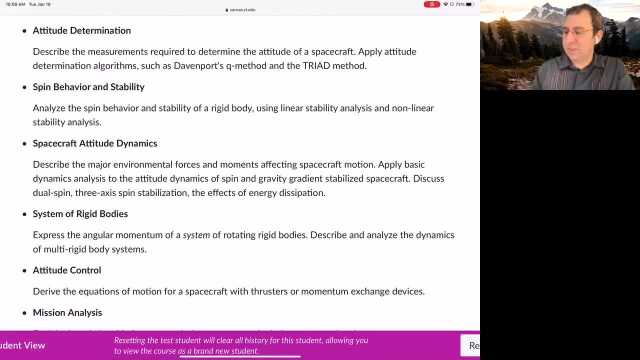 Then we get into some, how do you determine the attitude of something? So there'll be different measurements. There's sensors on board. 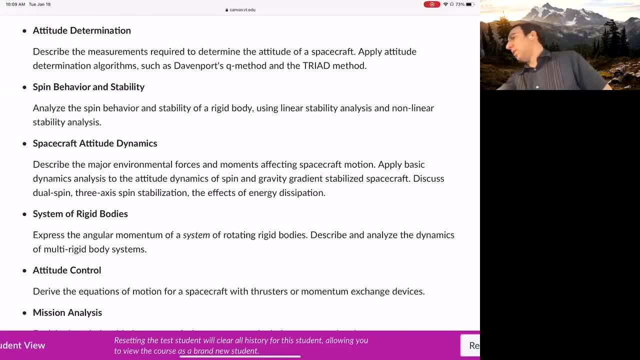 There's sensors on board. Our phones, all our phones have like tons of sensors. Your phone knows where it is with respect to the inertial frame. So your satellite should. 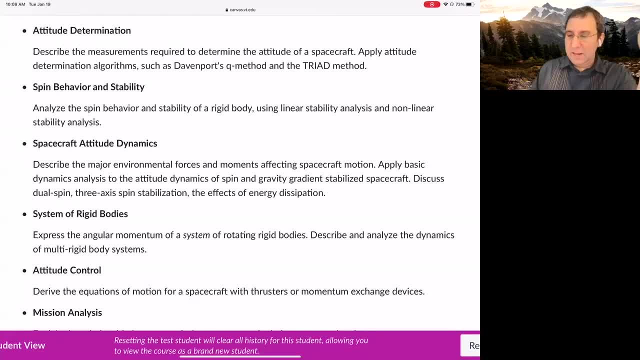 So your satellite should. There's spin behavior and stability. So there's the static, or I guess the uncontrolled dynamics of a satellite is what we're talking about here. 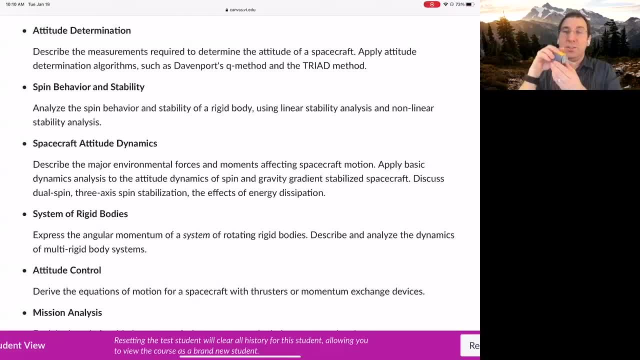 If you have a rigid body, are there directions in which it could rotate where it's stable. 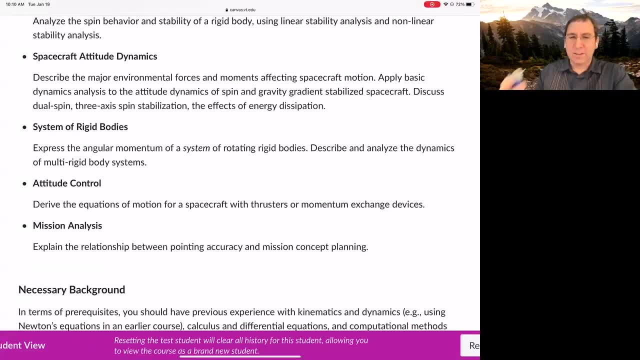 Spacecraft attitude dynamics, that just means taking attitude dynamics and looking at the environment that a spacecraft is in. 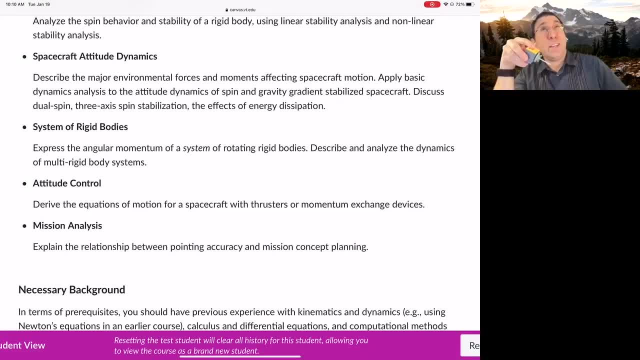 So environmental forces, what's the environment space? Well, there could be a little bit of drag. There's also, if you have a large enough body, then the gravity closer to Earth is stronger than the gravity further from Earth. And you could use that to your advantage. 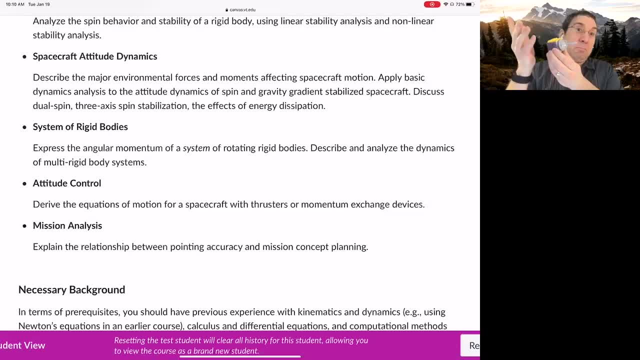 And there's also the magnetic field of the Earth. So we'll talk about that. 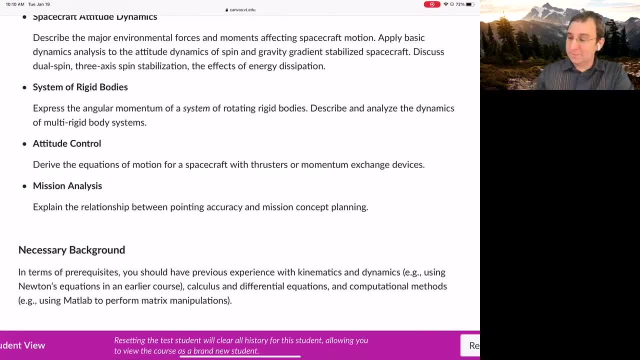 And then how to do control, some ideas about controlling. 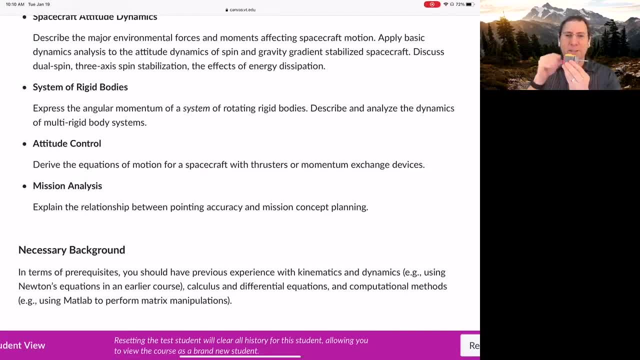 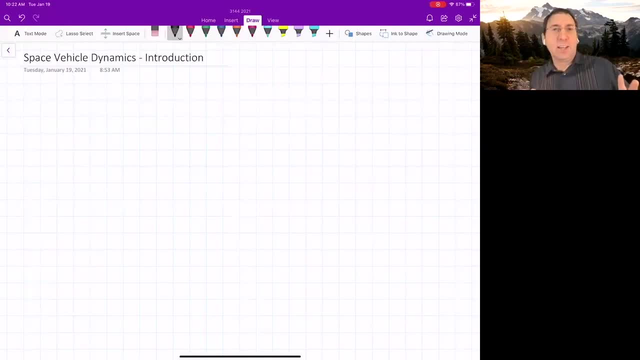 If you've got thrusters, you could turn something, or you could use momentum wheels. And those are less intuitive, but they're there. This is what most of the class is going to look like. I'm going to be on one note. With graph paper in the background. So it helps me draw straight, because I don't draw too straight. So let's just dive on in, OK? So the spacecraft attitude. 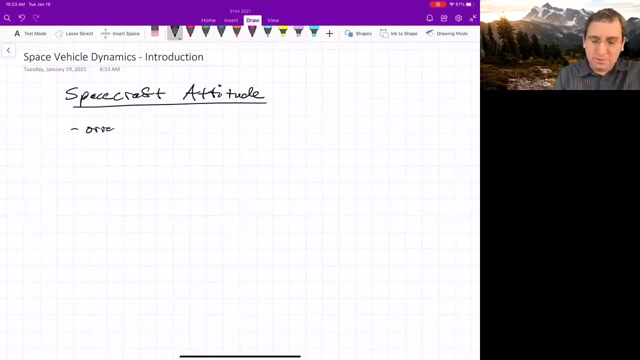 So this is just a sense of the terminology, the orientation, of a spacecraft, is called its attitude. 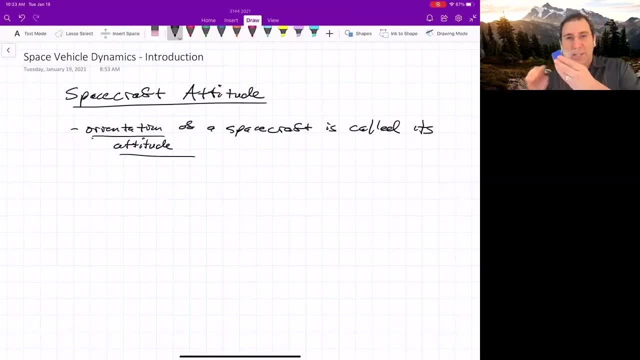 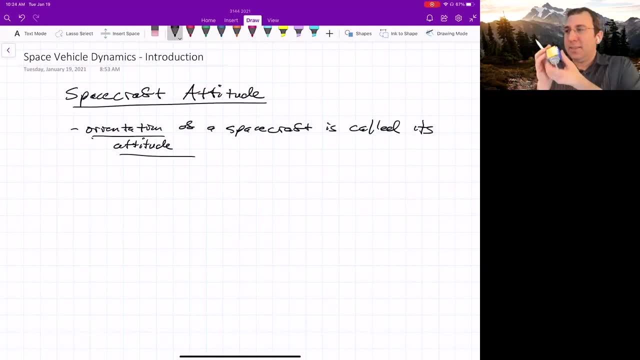 And spacecrafts have instruments and antennas on them that have to be pointed in specific directions. 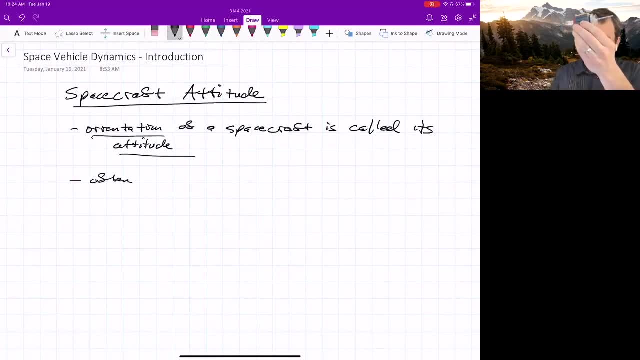 There's often instruments and antennas that have to be pointed in specific directions. 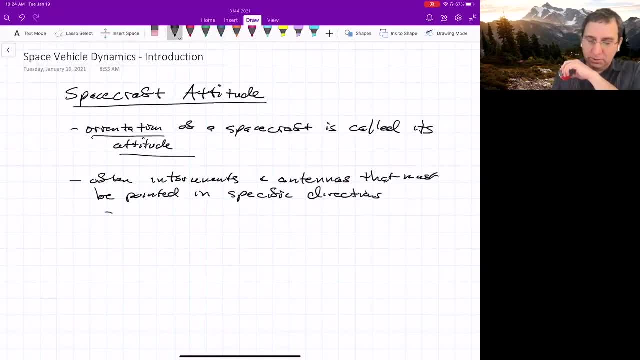 And they're always within some tolerance. So for example, the Hubble Space Telescope needs to point the telescope part, the mirror, has to point in the correct direction. The Hubble Space Telescope. 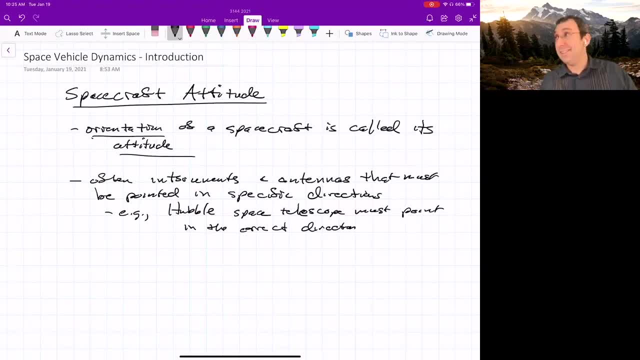 The Hubble Space Telescope also has the additional issue that it has to look at that thing and stay steady. Otherwise, the image will be blurred. It's like when you hold your camera and shake it. 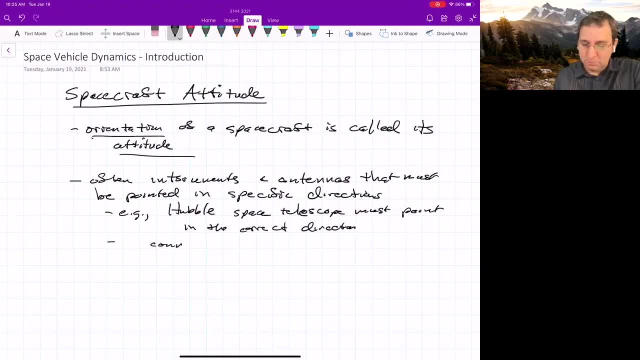 And then communication satellites have to point their antennas. 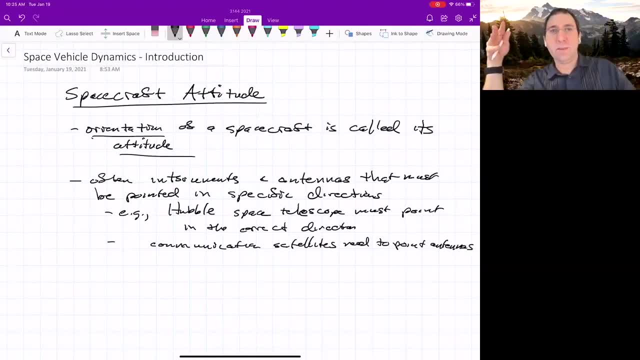 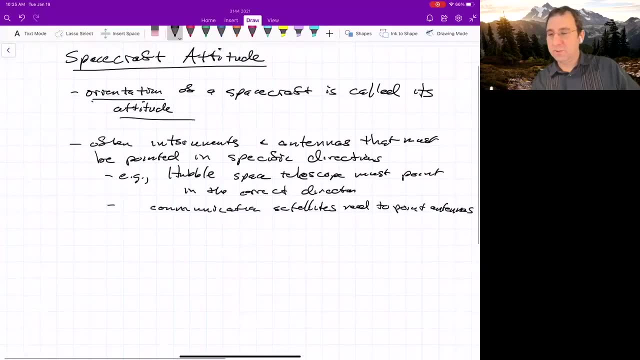 And now there's all this talk. About like giant constellations of communication satellites so that you could have internet access, internet anywhere in the world, thanks to spacecraft. 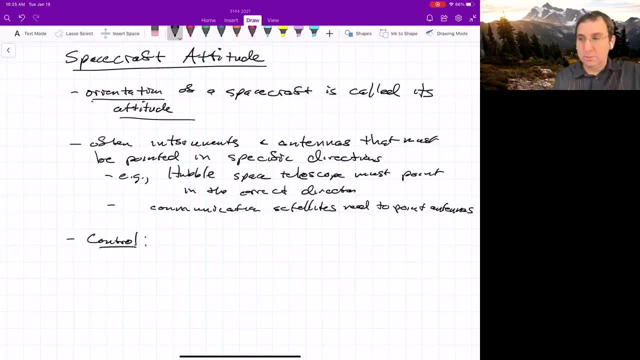 What about control? So to control the attitude, spacecraft operators, 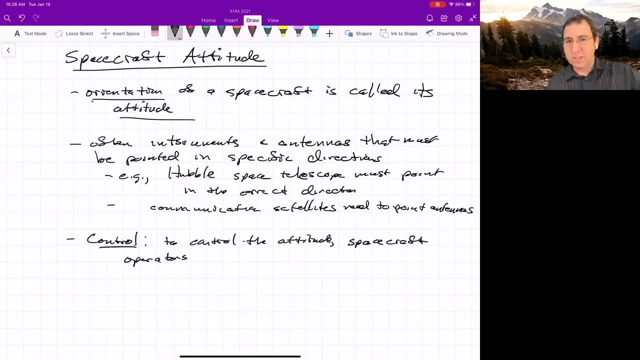 which could be the spacecraft's own computers, they must be able to determine the current attitude. Right. That's where sensors come in. And we can't do that. So there's an absolutely need for information. We can't have anything. 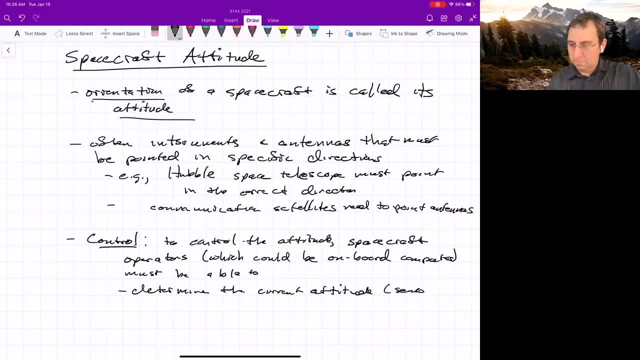 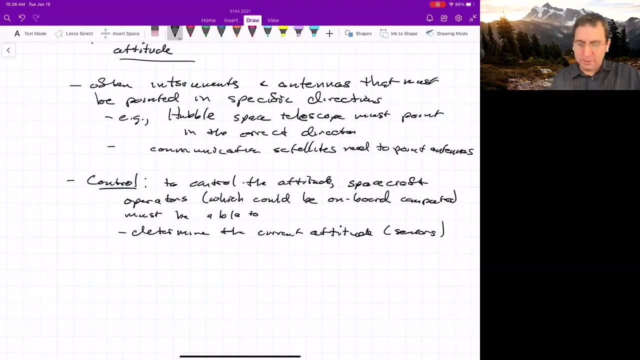 We can't have anything. Right. That's interesting. We have to realize that. We have to. And then determine the error between that current attitude and the desired attitude. 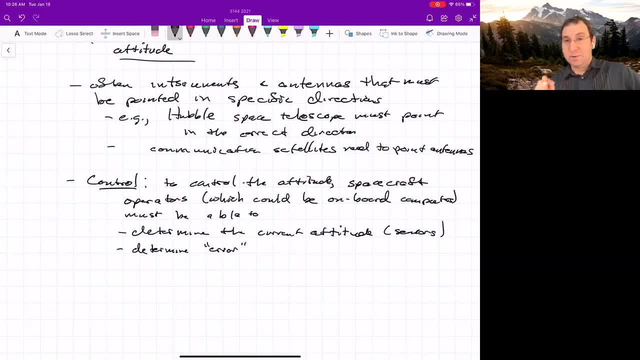 I kind of don't like calling it error. We just mean the difference between where you are currently pointing and where you want to point. 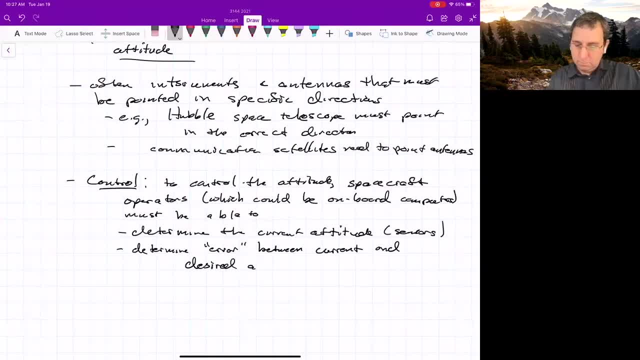 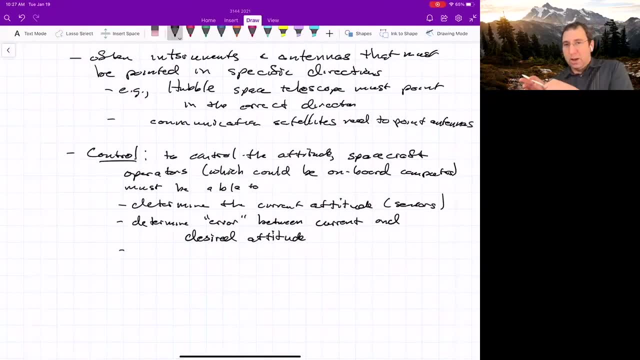 And once that's been determined, you know, how do you have to turn? Well, you have to figure out how you have to turn first, and then you would apply control torques. 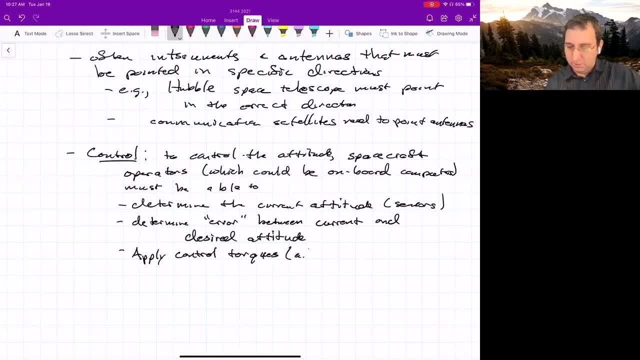 I might also refer to torques as moments. So anytime I just use torques. I'll use a different phrase. I'll put aka, also known as moments, control moments to reduce error to zero or close, close to zero. Right, nothing's perfect. Sensors always have noise. Actuators don't do things perfectly. Something. Something. 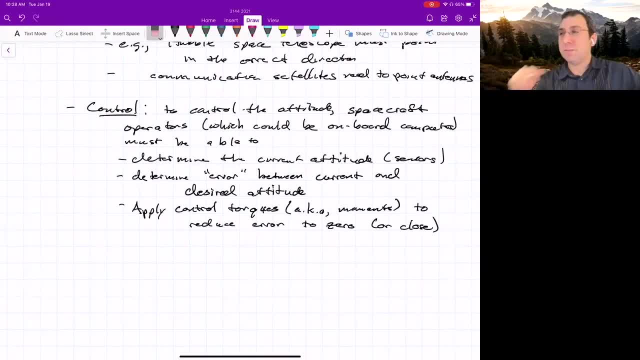 Sometimes the charge for the parachute gets put in backwards. No, we don't. Totally unrelated. All right. 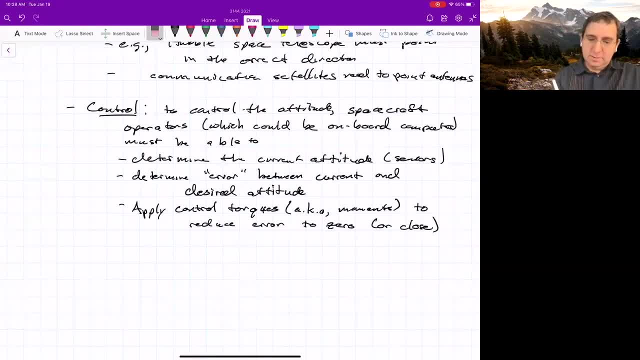 So the, that's just kind of, you know, broad. You've got the spacecraft. It's pointing in a certain direction. You want to point, oh, I have another vector. I have got a bunch of these little vectors. 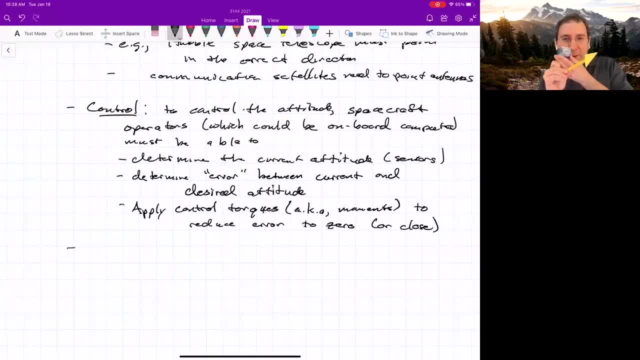 I want to point this way, and I'm pointing this way. So now I figure out, okay. I need to. Go that way. There. There are. 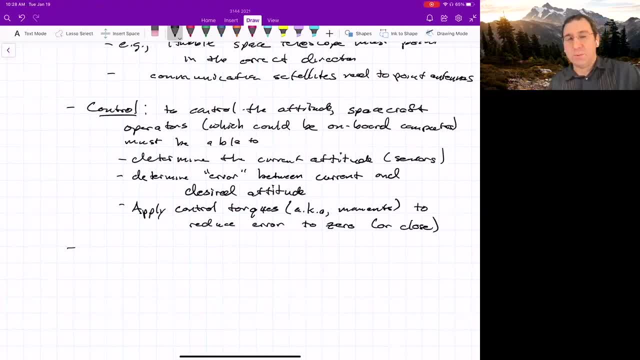 I guess I'll just tell you. There are coordinates that can describe the orientation of a rigid body with respect to a reference frame. And these are attitude coordinates. 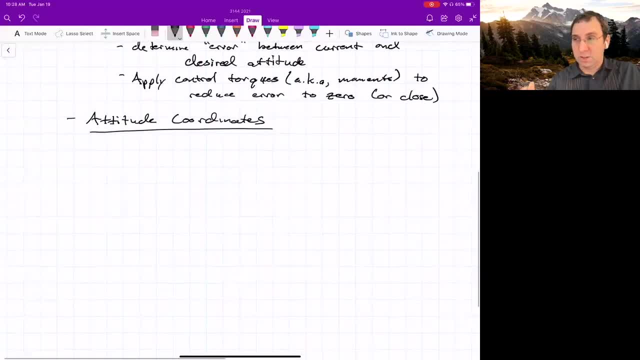 And there's different choices of them. We'll spend a lot of time talking about what should we use. 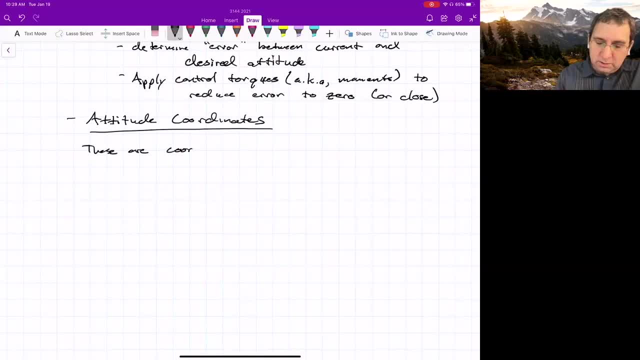 So these are coordinates. So these are coordinates. That completely describe. 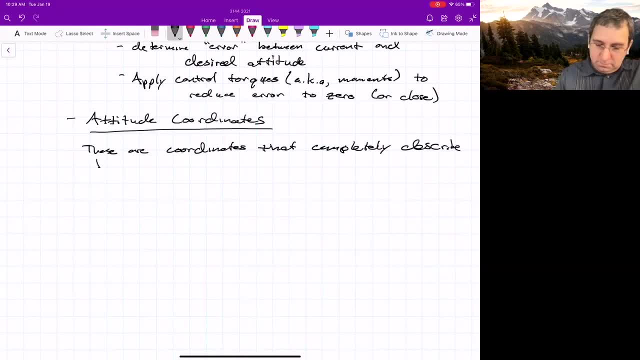 The orientation for rigid body. With respect to a reference frame. With respect to a reference frame. With respect to a reference frame. 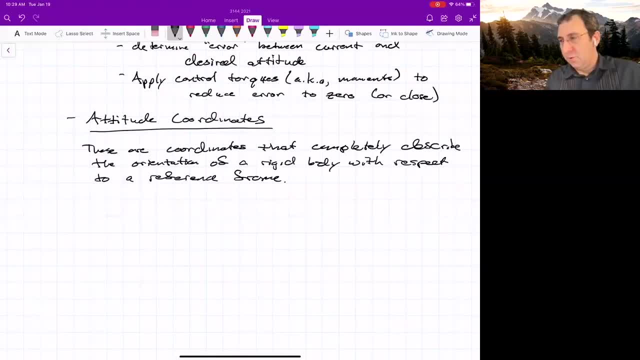 And by the way, I'm. And by the way, I'm. I often do not use PowerPoint slides because I've noticed sometimes I would blast through them quickly, whereas if I slowly write it out, you can see it. 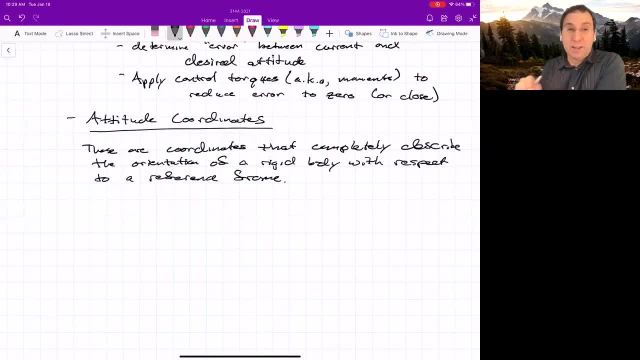 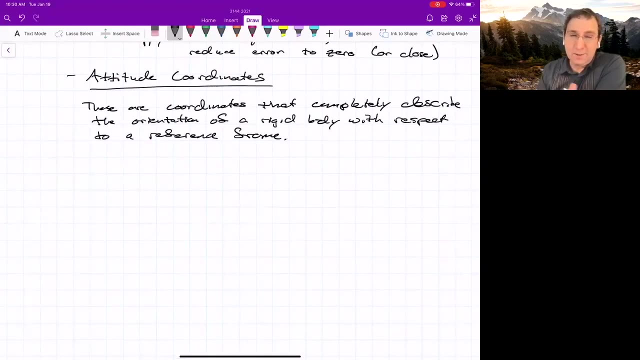 Plus, when I do work examples, I think it's much better for you to see me write it out. And for your own learning, it's probably good for you to take notes. And for your own learning, it's probably good for you to take notes. I'll say. I'll say. Even though this will be provided, it's good for you to take your own notes. 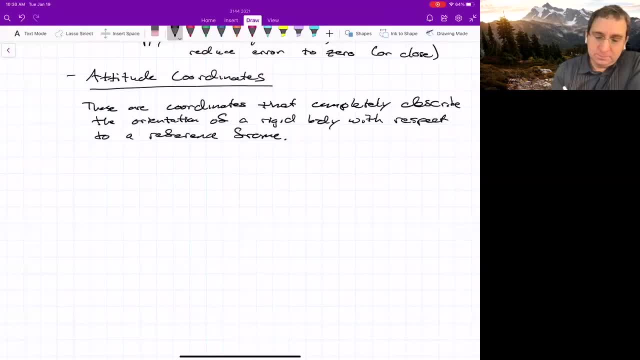 So to to define the attitude coordinates. 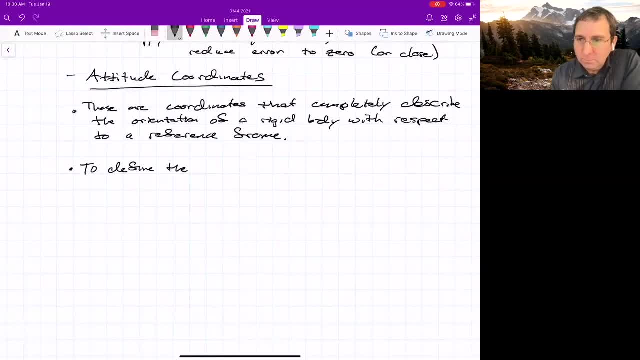 We have to select two frames. So there's a question. 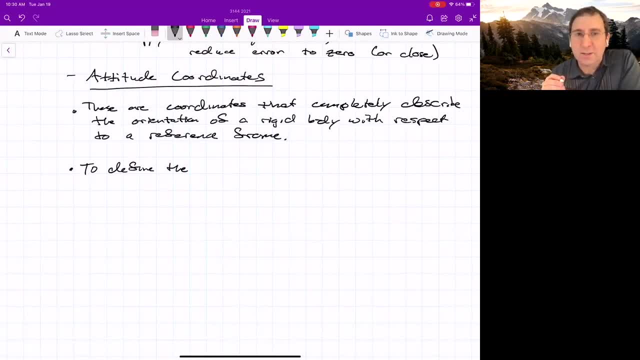 Do I give recommended readings from the book to follow along with the lectures? Yes, typically but. This stuff is not in the book. They don't really give like a high level here's what you. Why we're gonna do this. 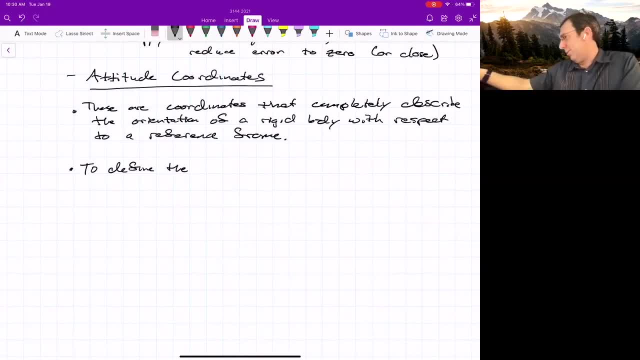 That so if you look at chapter one it kind of dives into particle dynamics. 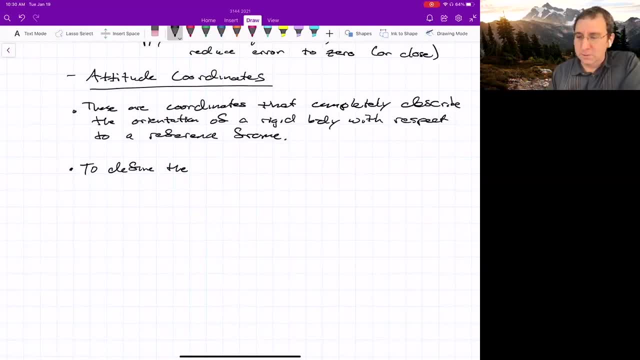 So unfortunately this isn't in the book but yeah I will try to give you know where to read the book. But yeah, I will try to give you. In the book. Where to read in the book. 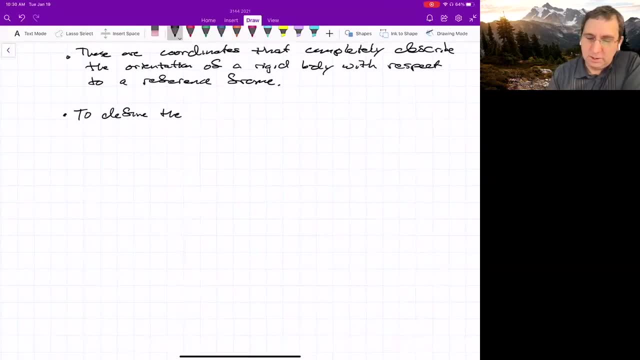 I'm so to define the at whoa. Whoa. OK. 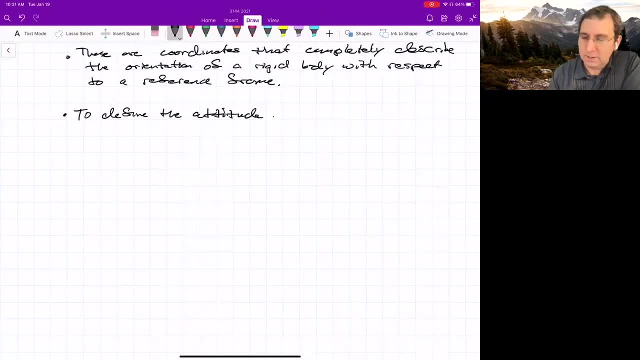 To define the attitude coordinates, we must select two frames. One is the frame to which the orientation is desired. 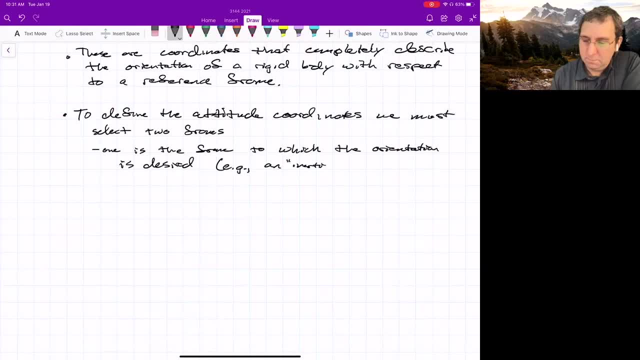 So for example, an inertial reference frame. 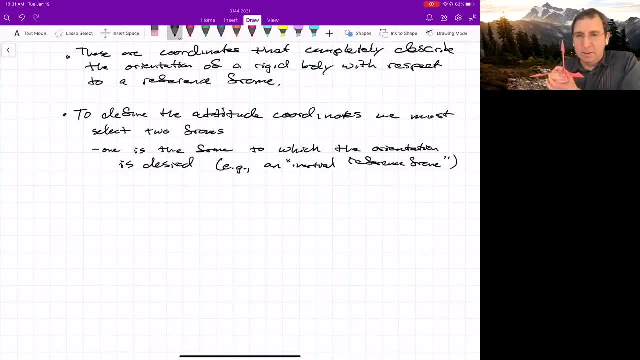 So I'm going to use the example of, here's an inertial reference frame. And I'll often actually use red vectors, because I have this red thing. So if this is my inertial reference frame and I've got a satellite, satellite will need to do something. I want this to be oriented in some way with respect to this inertially fixed reference frame. So this first thing would be the inertial reference frame. The other one needs to be a frame attached to the body. 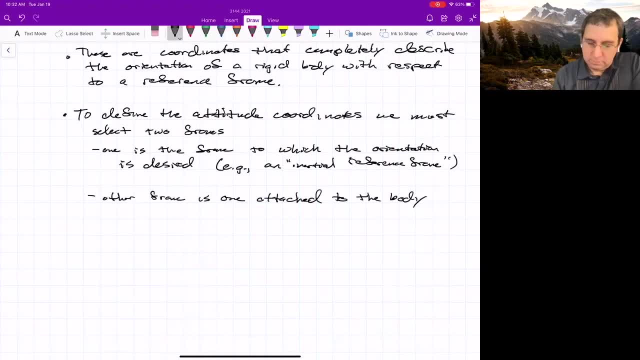 Attached to the body. Often called a body fixed reference frame. 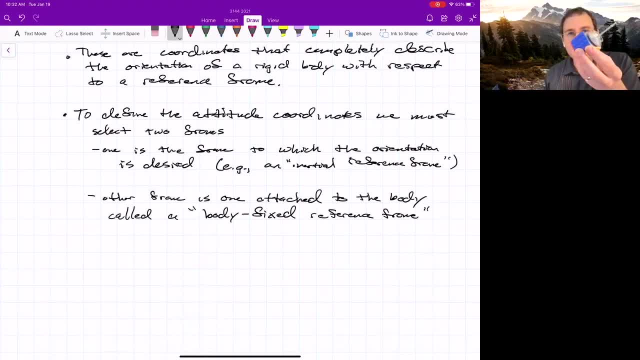 So if this is my rigid body, it's a satellite, I would attach a frame to it. And it's like, this frame is attached to the body. So now I can kind of abstract away. I can take the body away and it's just, okay, I have the, this is a body fixed frame. 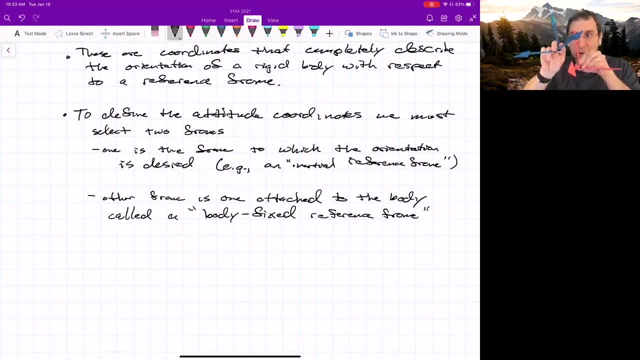 And how do I describe the orientation of this blue frame? I keep calling it a frame. 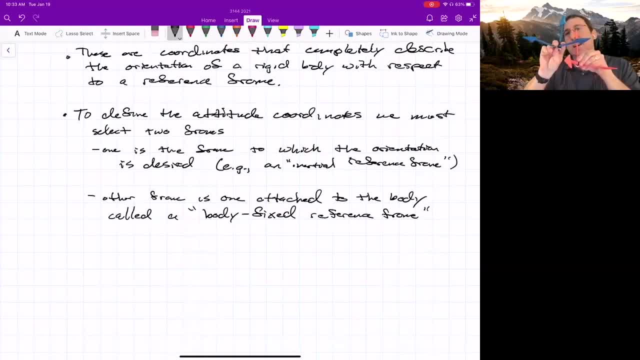 It's a triad of unit vectors that describe a right-handed coordinate system. One is attached to the body. One is the inertial frame. How do I describe the orientation of these two? Well, that's what attitude coordinates are. 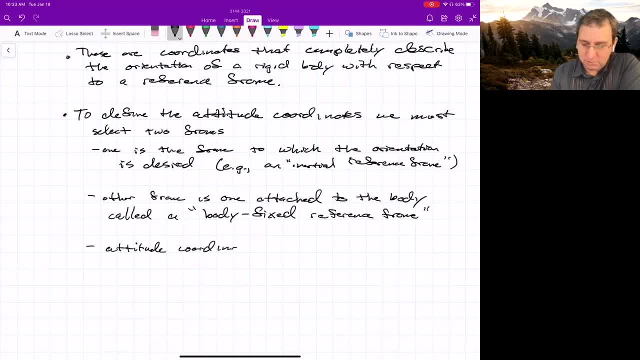 So attitude coordinates relate these two frames. Okay. Okay. Okay. Okay. Okay. 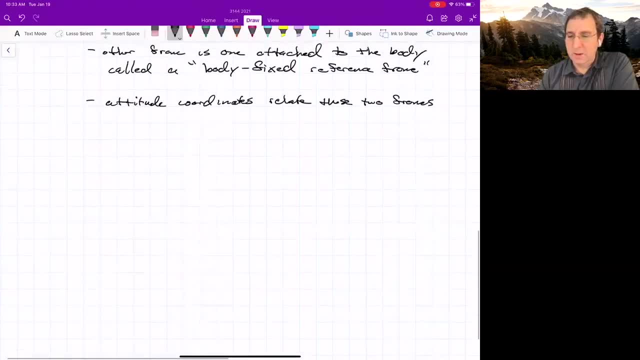 And just some points that maybe aren't obvious. 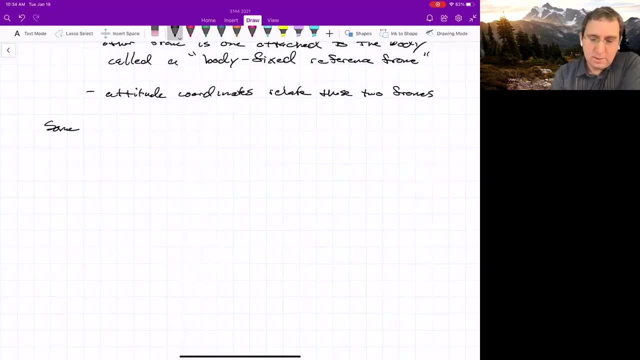 And we will go into more detail about this later. 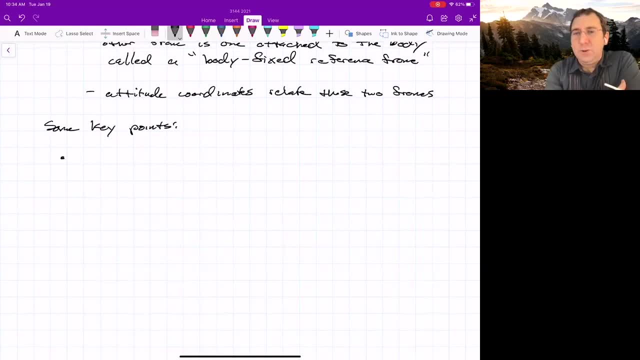 You need at least three coordinates to describe the orientation between two frames. So that means that you need three numbers. So you need at least three numbers and it may be not, it's not obvious, but just to roughly tell you, what are these three numbers mean? We got these two frames. 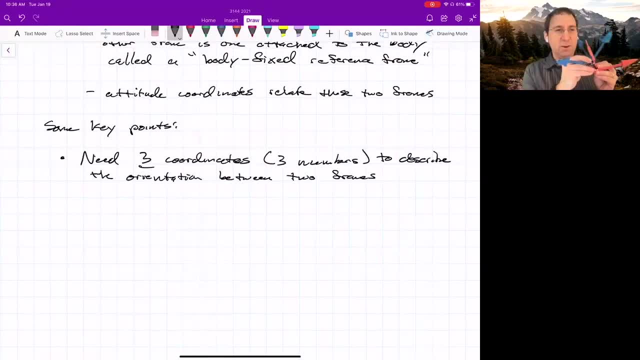 If I want to describe like an arbitrary orientation of one frame compared to another, I can do a series of three rotations about primary axes. So I would rotate a certain angle. I would roll through one and then a certain angle through other and a certain angle through the other. 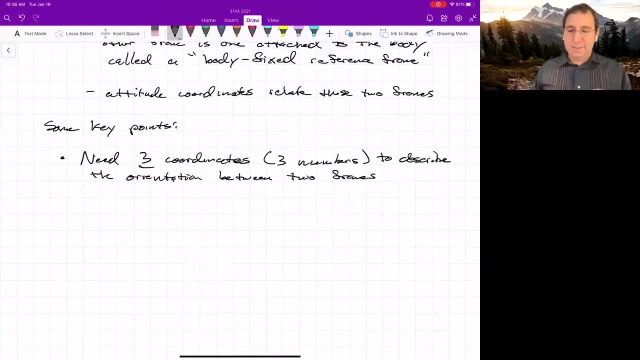 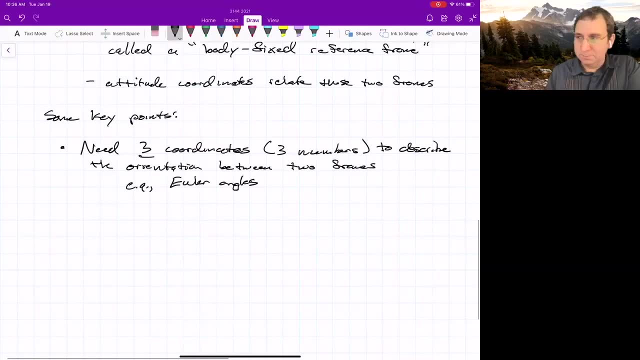 So three numbers. So there's a, these are called Euler angles. The typical ones that you've probably heard of, and they're just one set among many, are yaw, pitch, and roll. 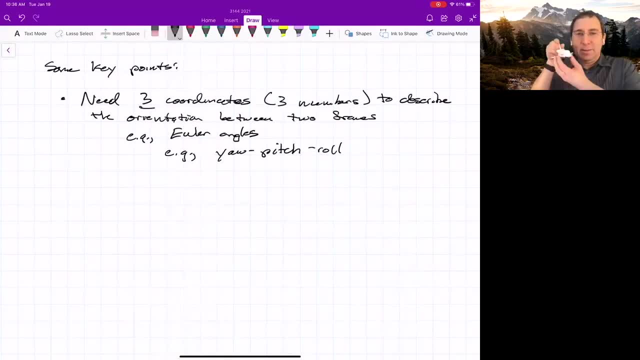 Okay. And then if you combine those, like a yaw, a pitch, and a roll, you can define an arbitrary orientation of the space shuttle compared to an inertial frame. 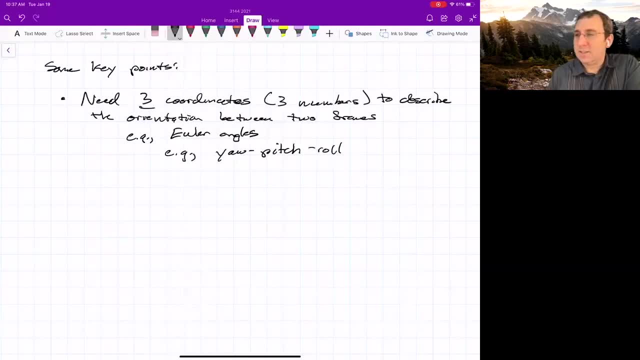 Now, the problem with using just three coordinates is that if you only have three, Now, the problem with using just three coordinates is that if you only have three, there's going to be at least one orientation where the coordinates are called singular. So, if only three coordinates are used, this can lead to problems. And that's why even though they're nice for explaining things, they're often not the ones that are actually used for spacecraft. 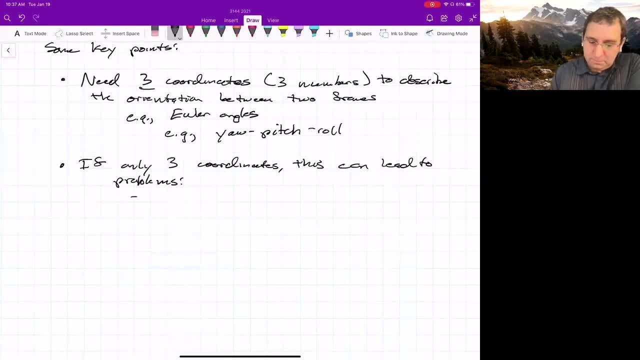 what is this problem? There will be at least one orientation where coordinates are singular. 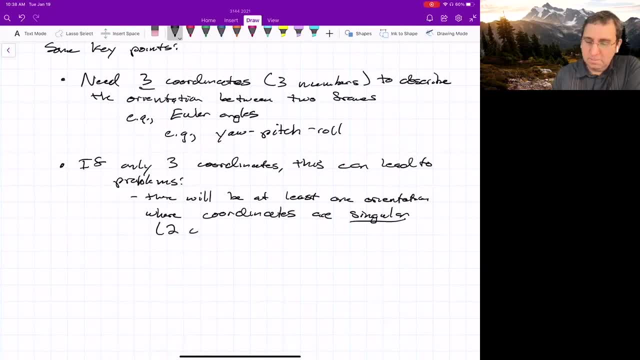 You might be, okay, what does that mean? That means, okay, two coordinates are undefined or not unique. 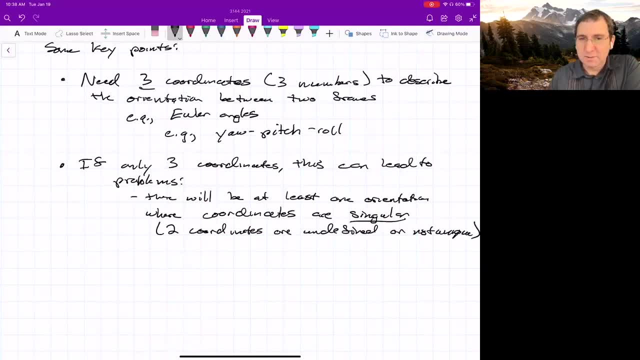 I mean, just think of singular as bad. The singularity, the middle of a black hole, you don't want that to happen to you. 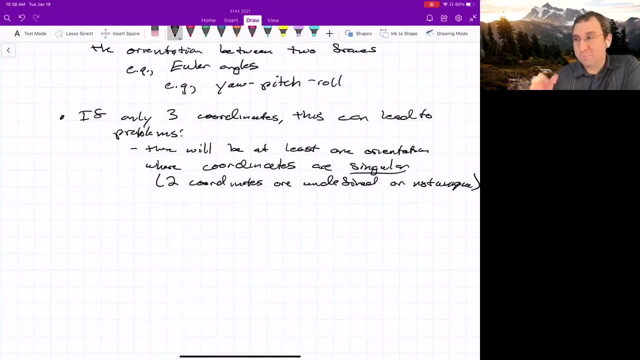 All right, so at this, at those orientations, these problematic or singular orientations, there are some differential equations that also lead to, problems. 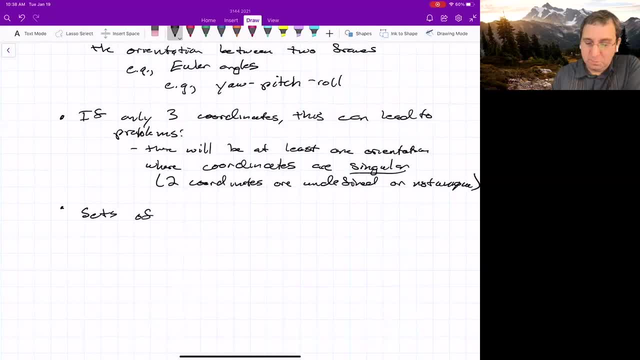 So people have come up with sets of four coordinates. 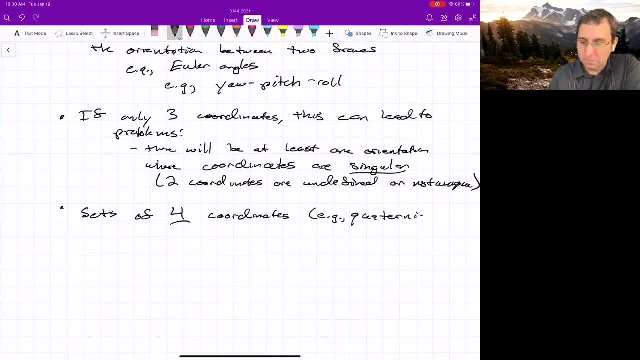 For example, things called quaternions. And there's others. 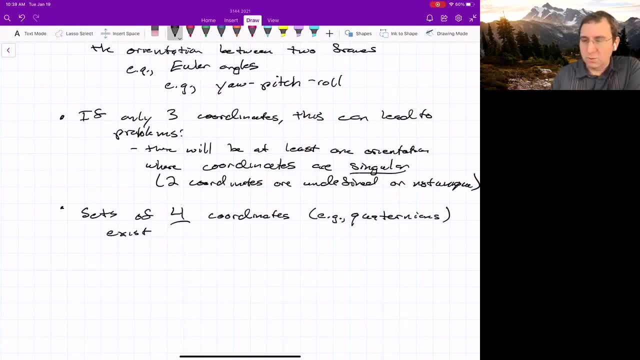 There are sets of four coordinates that exist which do not contain singularity, so they don't have this problem. 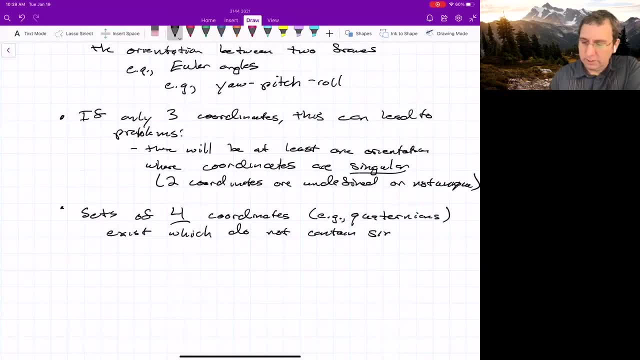 And maybe you're asking, like, who cares? If you've ever seen, you're playing some video game and the orientation of something just goes crazy. Maybe they were using Euler angles and it went to one of those singular configurations. 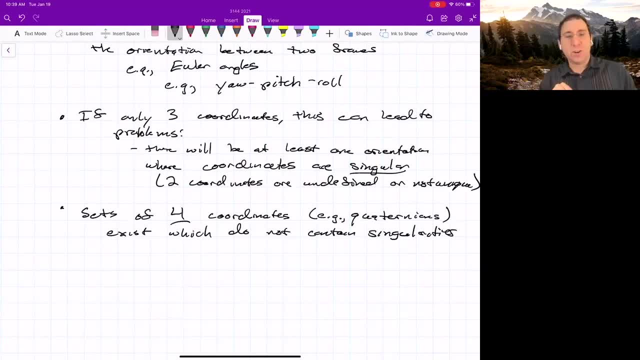 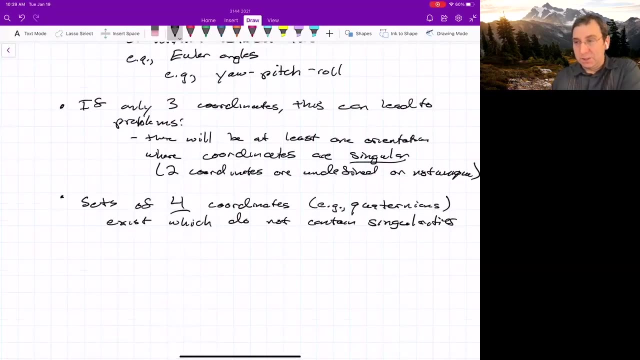 Numerically, something will, a one over zero will occur. And then, you know, the computation stops. So you don't want that on a $200 million satellite. So there's sets of four coordinates that do not contain these singularities, but the coordinates are not independent. They're constrained by, constrained equations. All right. So, hold on, hold on. 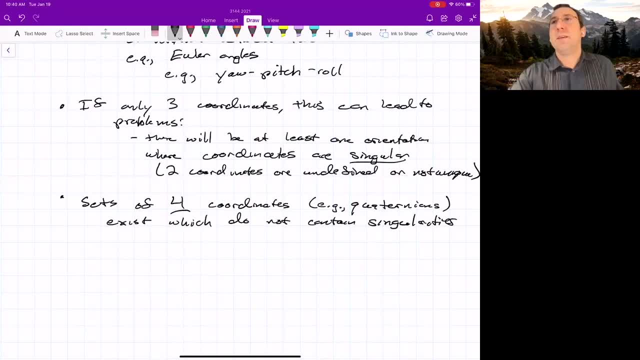 Let me draw, I haven't drawn any pictures. Like, what's up with that? Uh, it's a bit confusing, but let me see. I think I got it. All right. Here we go. 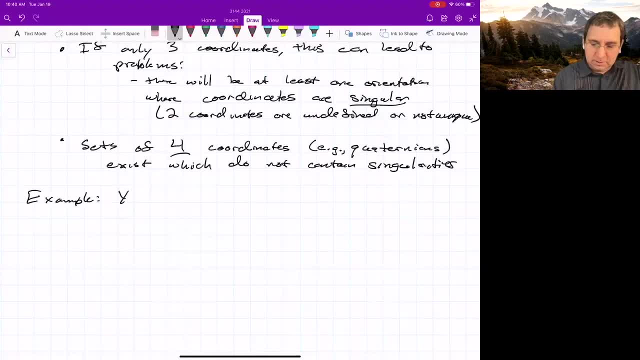 So, the example of, let me say yaw, pitch and roll. 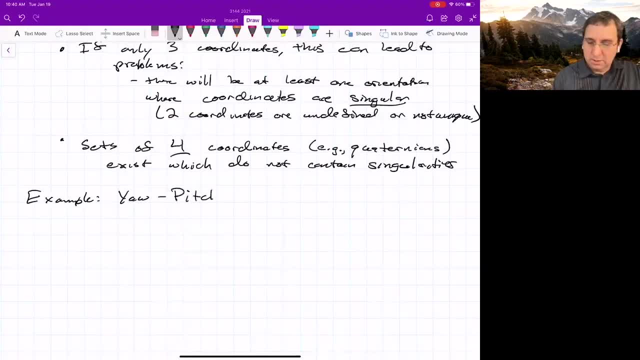 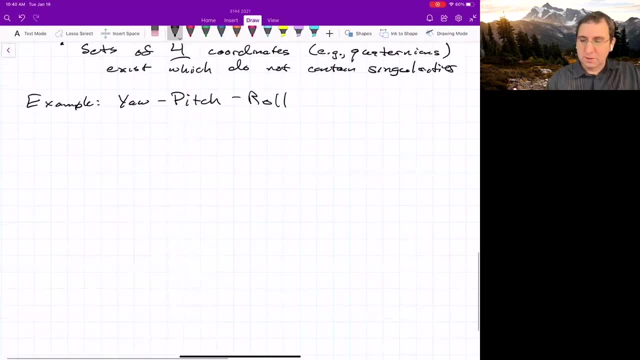 So, the example of, let me say, yaw, pitch and roll. So this is often used with aircraft. 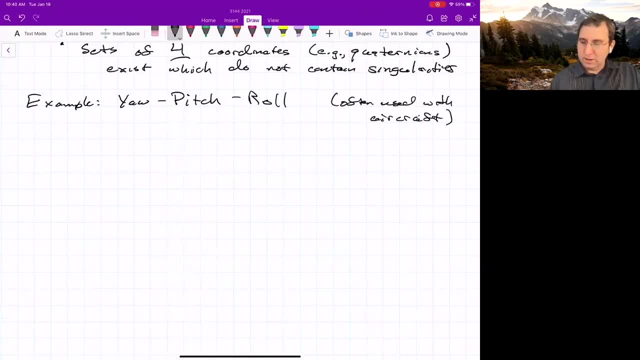 if you've got a try to draw here's the this is earth gosh that's terrible looking that's that's earth okay there's earth and there is a frame attached to the earth we could call this the i'll use capital i capital j capital k so this is the this is the earth centered inertial frame 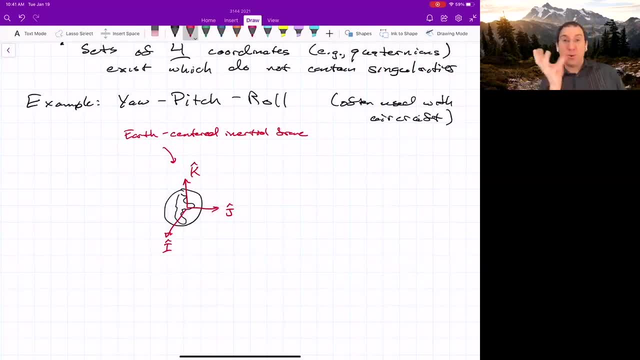 and it's right the earth is rotating with respect to this frame so let's say this is the earth centered inertial frame where we'll get into more detail later about what these directions are but this is a set of directions that as newton would have said are fixed with respect to the stars the distant stars he didn't think the stars were moving we now know they are but you've got a frame oh my goodness i have an earth here wow i don't know if i'll use this much you there's green ones and i have a green screen here so green countries just sort of disappear ah so the earth is rotating with respect to this inertially fixed frame 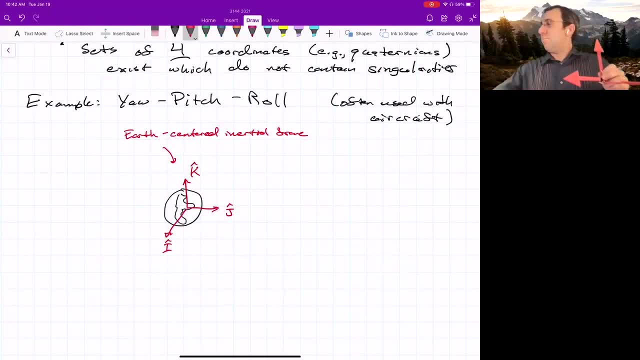 but this inertial frame is to give it a centered at the center of the earth and does not move with respect to the distant stars and then we've got our spacecraft and i don't know how to draw a spacecraft here's a spacecraft looks like a box and we'll put a frame on this actually here's the spacecraft 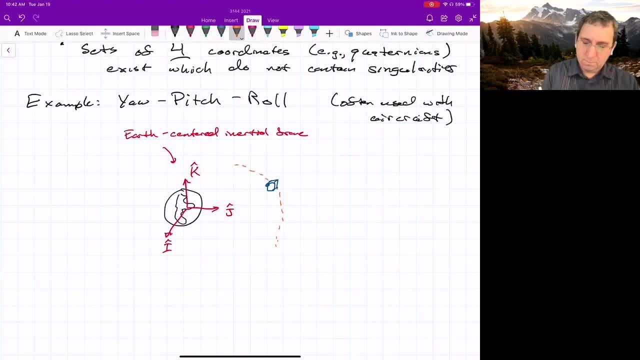 and it's in some kind of orbit right this is the spacecraft i don't know what i was drawing there spacecraft orbit just a little piece of it and often thanks to delta jump we've found a solid and even one sideく if you are into linear 좌z an朱 or maybe you don't get what i'm talking about locals who have this big long planet and they try to find small and big Grav gan Onionける One will describe a frame for the spacecraft orbit. 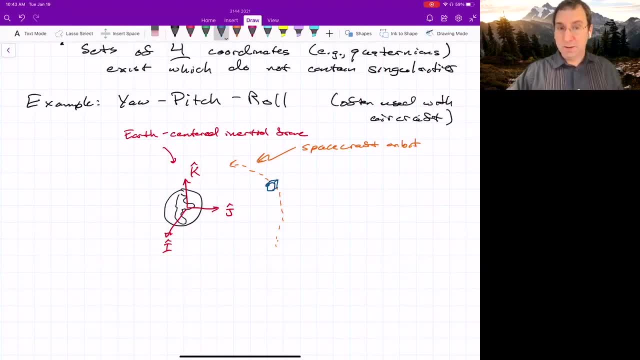 But right now, we're just going to write a frame for the body. So suppose this is our box. And I'll use blue because I've got this blue frame. Suppose I've got, I'll call this B1, B2, and B3. 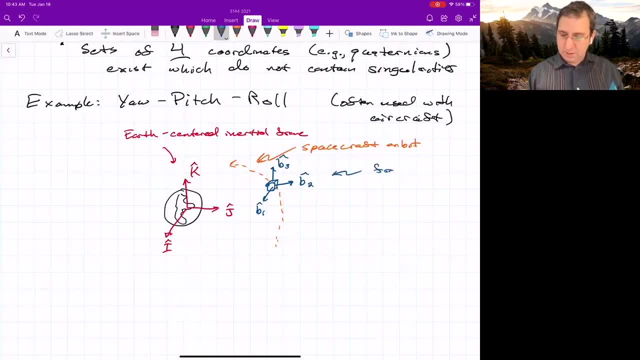 And this is the frame attached to the spacecraft. 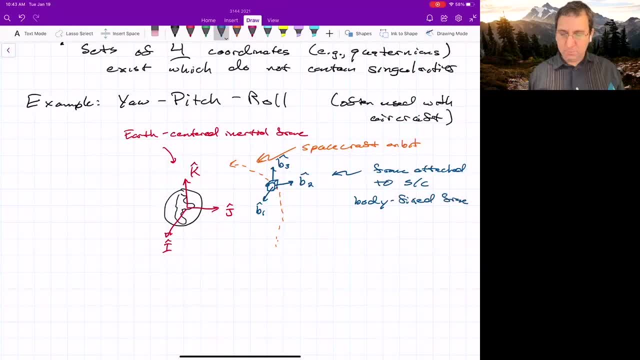 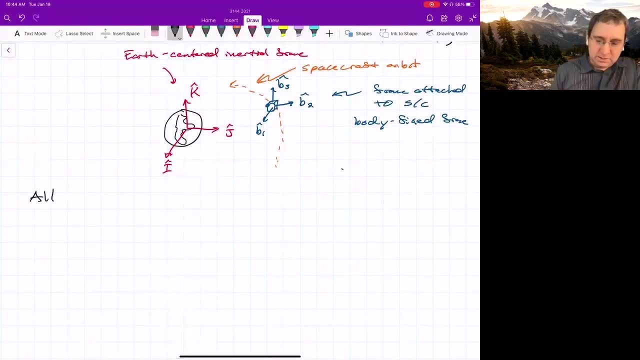 So it's a body fixed frame. In the last minute, let me just say something about all spacecraft need an attitude 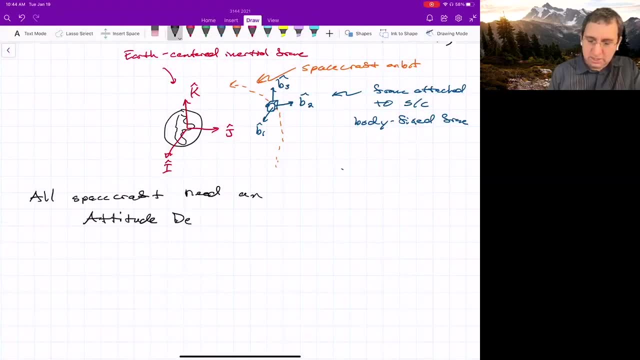 of determination and a control system. This is often abbreviated as ADCS. It's not just spacecraft that needs these. 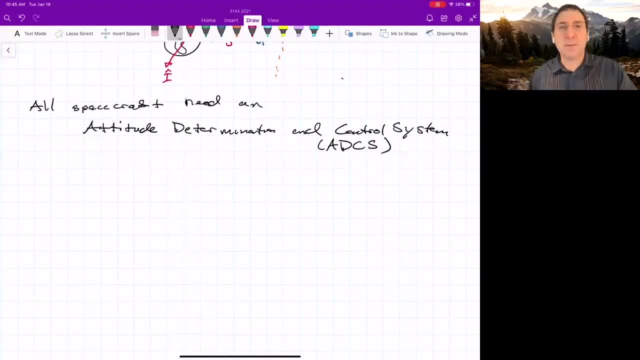 A drone, that I will later fly today, will need one of these. So there's math involved in the determination, and control system. And you can do this. And you can do that. 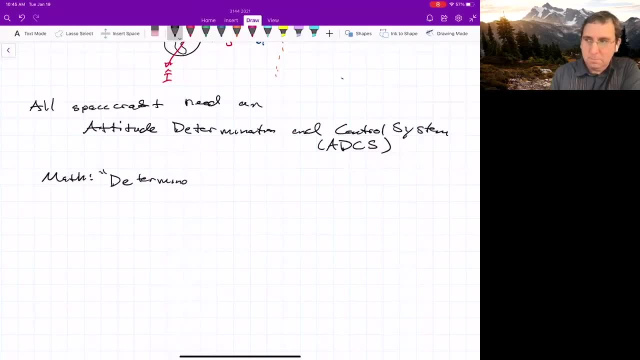 determination. Determination requires knowledge of kinematics. The math part. Technology is that determination requires sensors that are up to the task of doing this. And then the control part in this attitude, determination, and control. Control requires knowledge of dynamics.